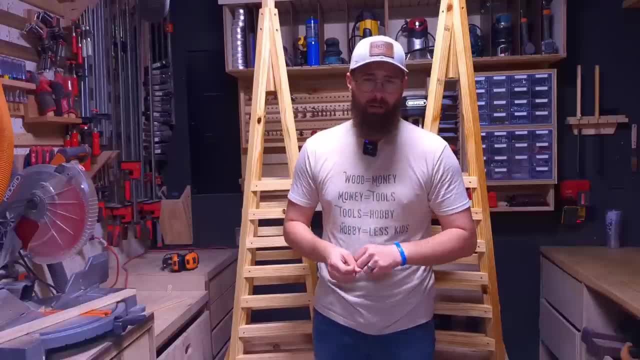 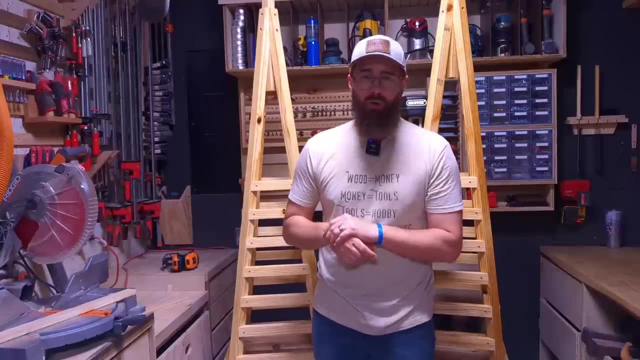 I will make a community post with a link to my website where the plan will be. If you want to be notified, you should make sure you subscribe, hit the bell icon and as soon as I post them you will know. I will also update the description that will have a link to the plans once I have it. 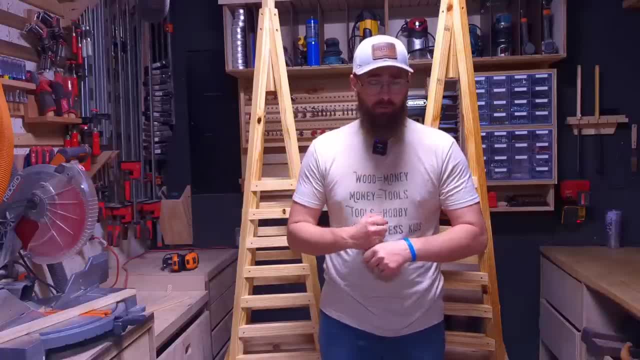 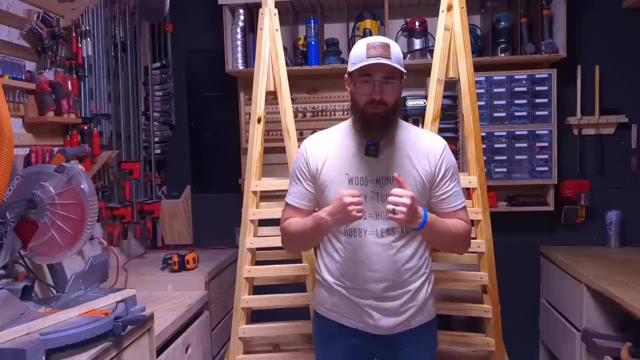 finished. Anyway, let's start talking about this build. So this is an easy, easy project that's selling very well in my area. One thing I'm going to talk about is the plan, So I'm going to talk making sure to focus on doing is test the market before I make a video on these and tell you that. 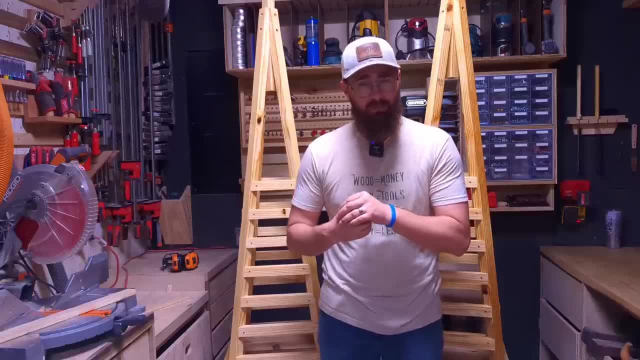 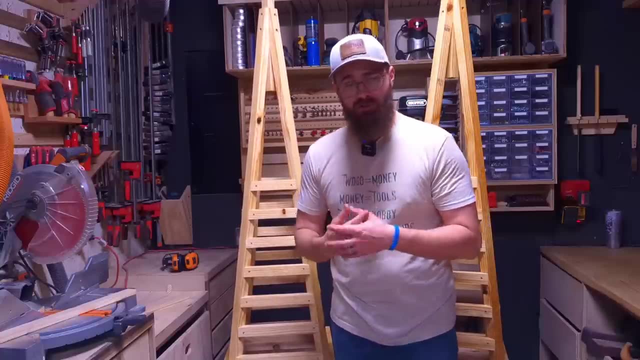 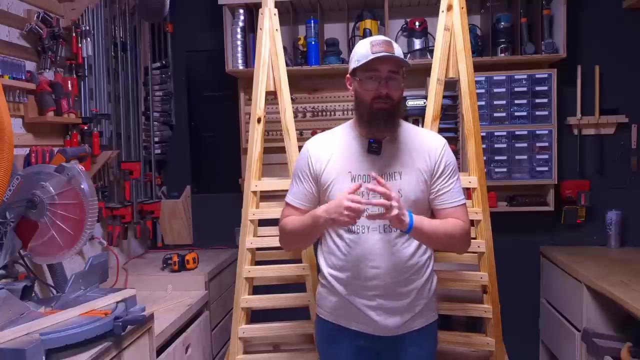 they sell. I make sure that they sell by posting them and selling them myself. So I have about $35 expense total in each planter. Five, two by sixes from the big box store, which are $4 and 32 cents currently in my area. A little bit of finish, a little bit of screws and that's it, A couple. 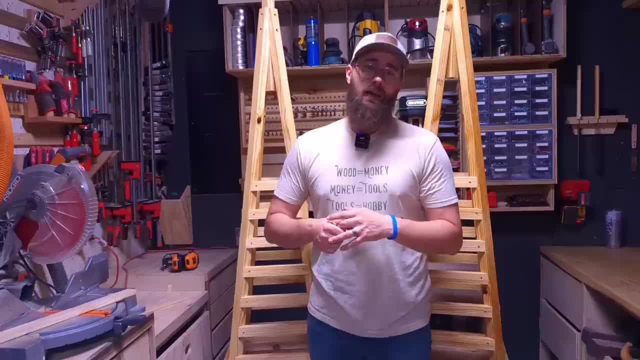 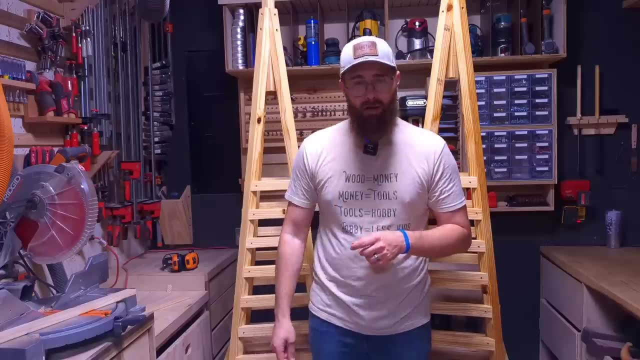 hours of work. That's really all there is to it. I'm selling these for $200 for one, or $300 and $350 for a pair of two. A pair is two. I don't know why I elaborated that, but it is. 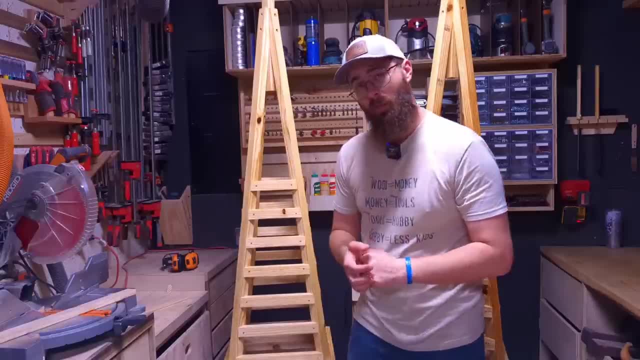 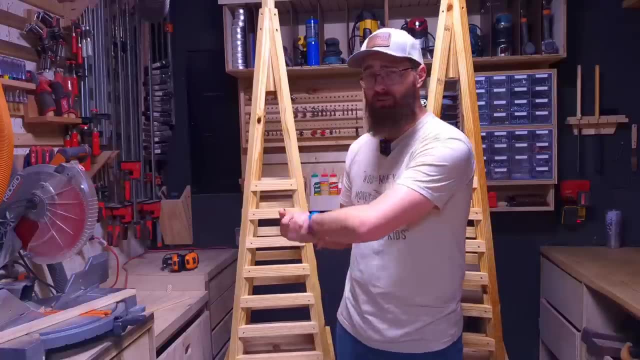 considered elaborated, You're welcome. So pretty good profit margins, eh, Pretty good profit, Even if you're paying yourself for your time and you consider your time valuable. these can be done in about an hour and a half to two hours per theater. Make a profit, You're. 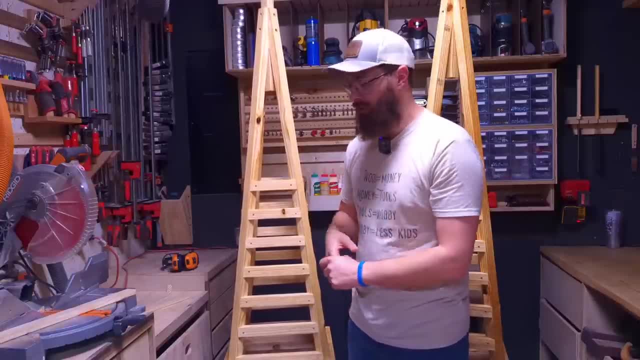 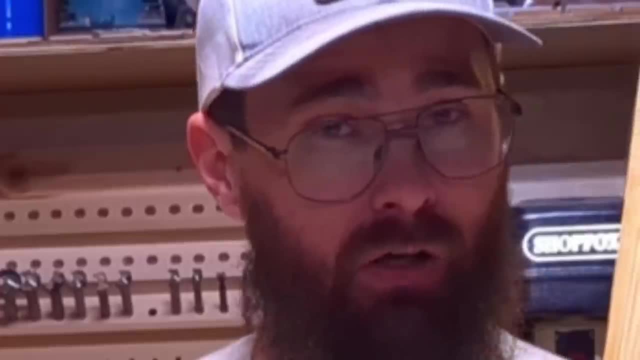 still paying yourself. You're still covering your expenses. It's a good project, Very easy to sell. Within two hours of posting we had two of them sold Now I made them and now we're getting rid of them. That being said, let's get started. 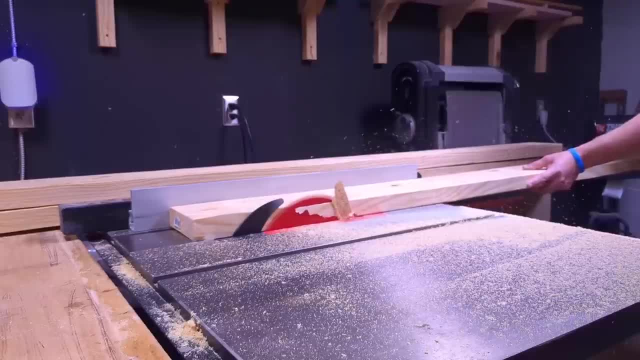 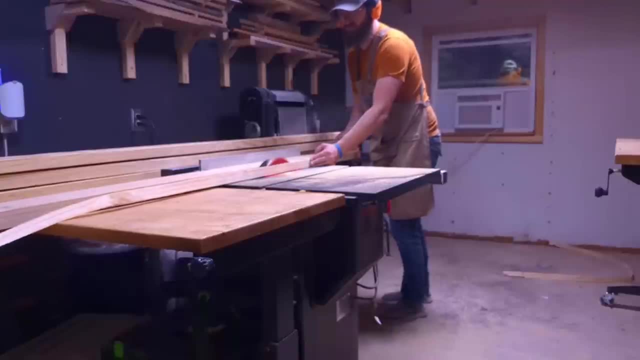 running through the cut list. So anytime you're dealing with dimensioned lumber, you want to make sure you take off the round over, And that's what I did. I took off the round over off of every two by six, and then you use that flat edge for the reference. 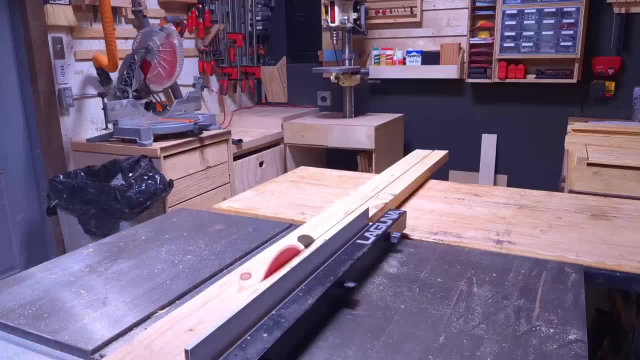 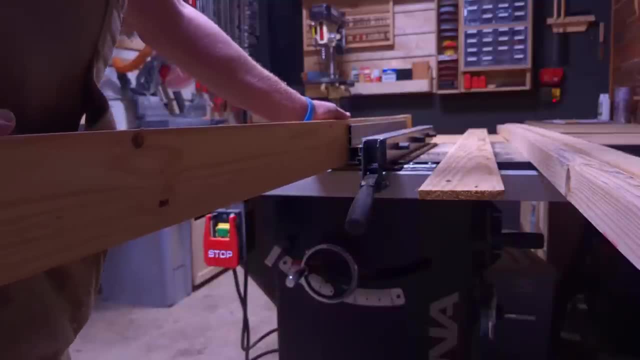 Right now we're just running through the cut list. I'm cutting out these one and a half inch strips. Those will be used for the legs and the aprons, And right here I'm ripping down or resawing the wood for the panel. So we'll actually make. 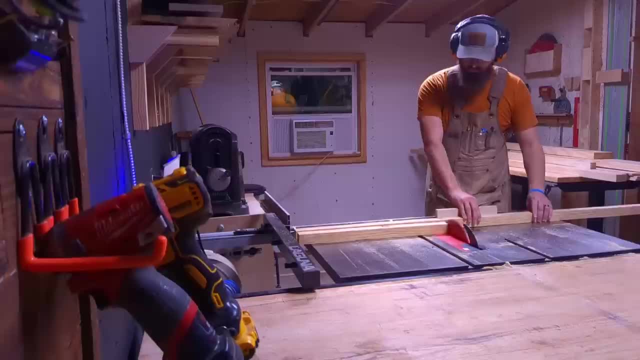 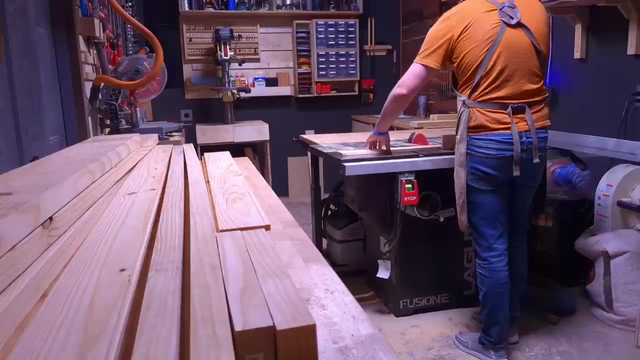 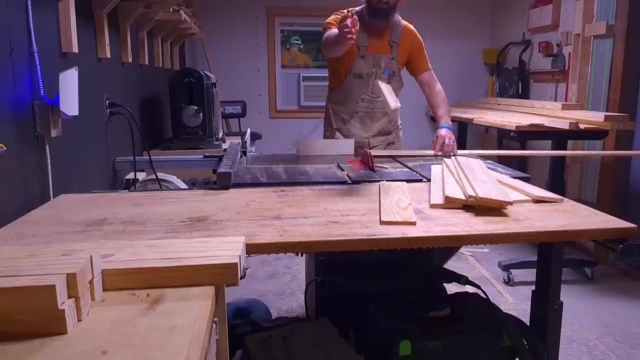 shiplap out of this. I prefer to do all of my cross cuts on the table saw. I'll do as many as I can, because it's just more accurate in my opinion. I can set the fence. Once it's set, all the pieces come out identical. So here we're, cutting down the shiplap or cross, cutting these to. 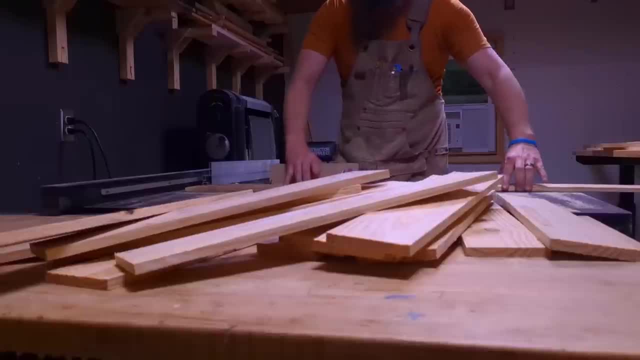 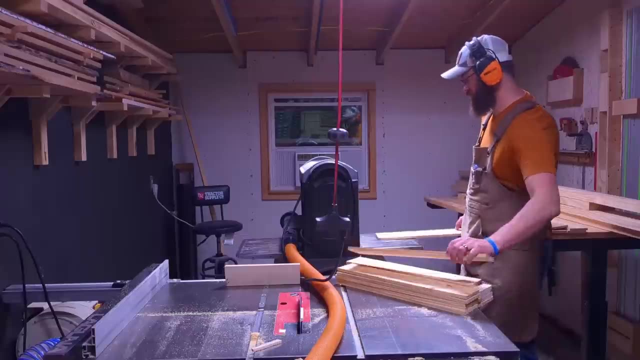 length Here. shortly we're going to start cutting the grooves for the shiplap. It's not a complicated process, Very easy to do, And I did it with just a single saw blade. In case you don't have a dado stack, you can do this without. 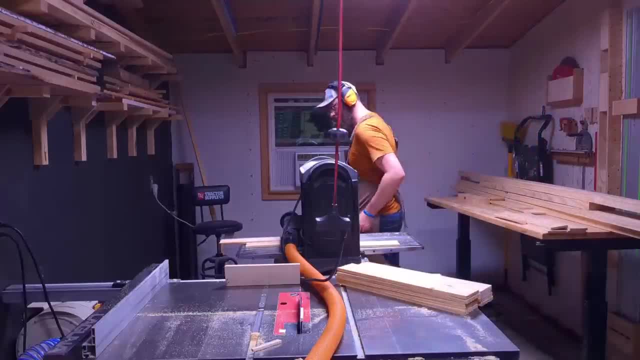 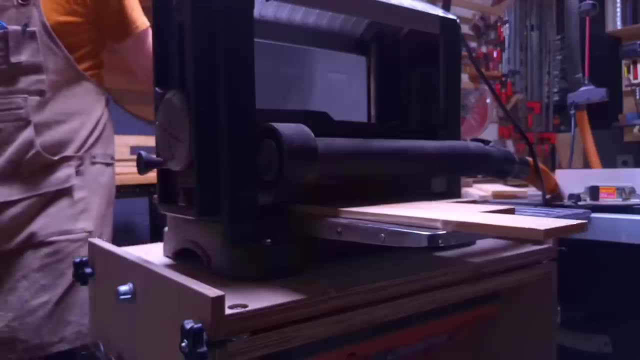 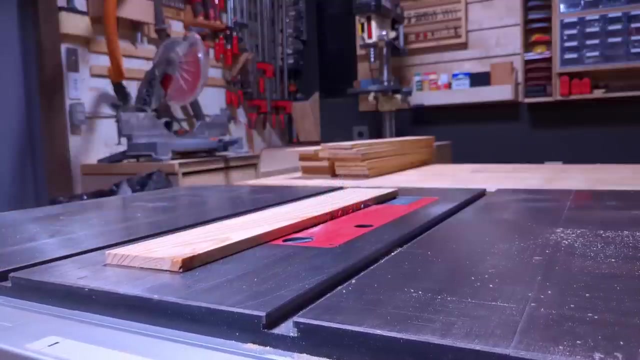 a dado stack, And so I'm barely taking off an nth of a degree, really just taking off the writing that's on these pieces of board. You know how they stamp it: the dimensional lumber. So I'm taking that off on the planer. So don't do a lot of sanding on this project. So here I'm lowering. 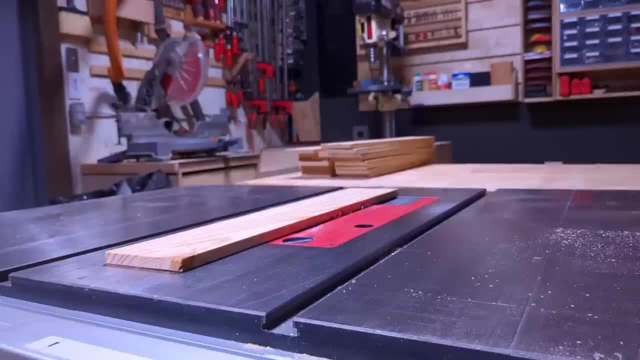 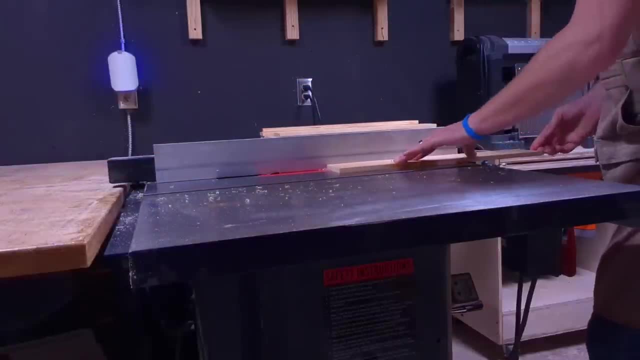 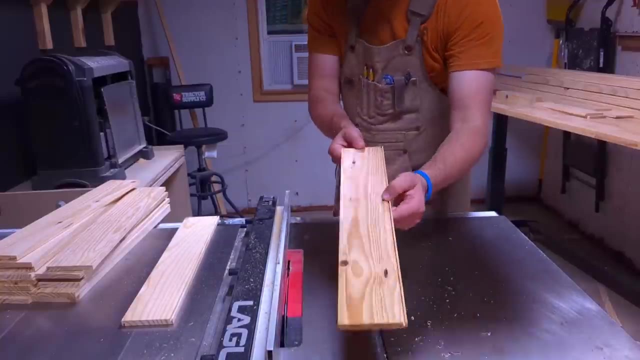 it. I'm going to start doing the shiplap and it takes a couple of passes. So this should be lowered to about half the thickness of your shiplap piece And you're going to go in an eighth of an inch wide shiplap, So an eighth of an inch wide by half the thickness. deep Now I accidentally went. 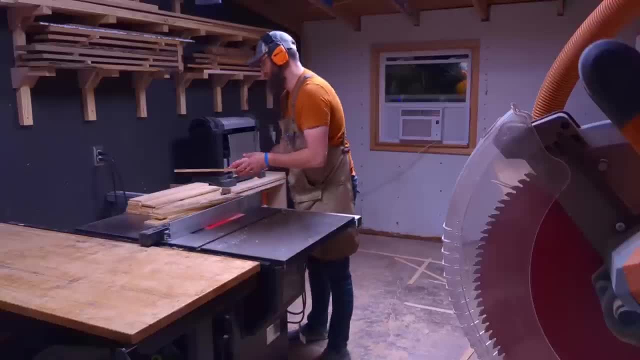 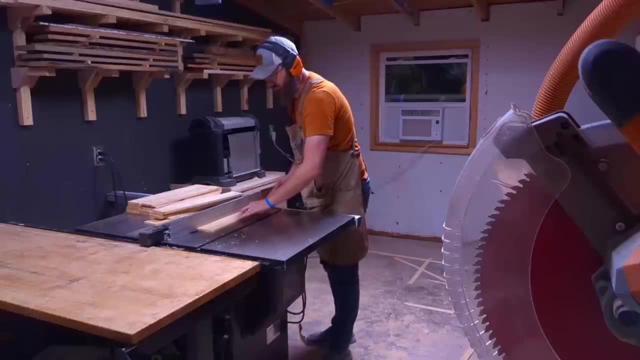 a little bit too wide on this one. I actually went a quarter inch. I wasn't paying attention So I had to accommodate the aprons. I had to cut those down a little more off camera To make this planer box work, But it just takes a couple passes. You slowly go towards that outside. 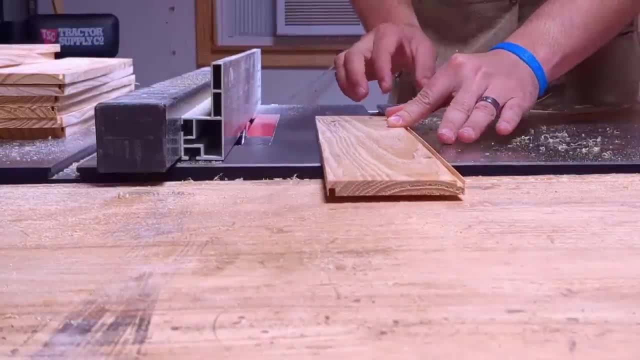 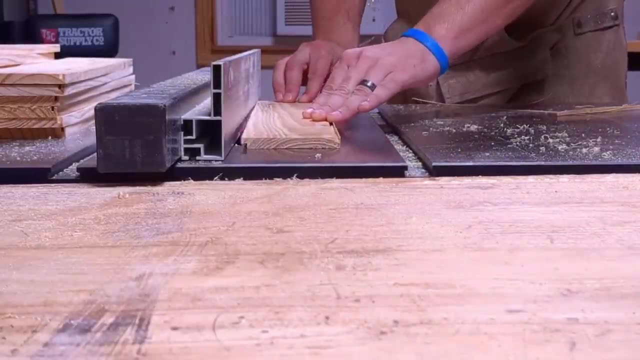 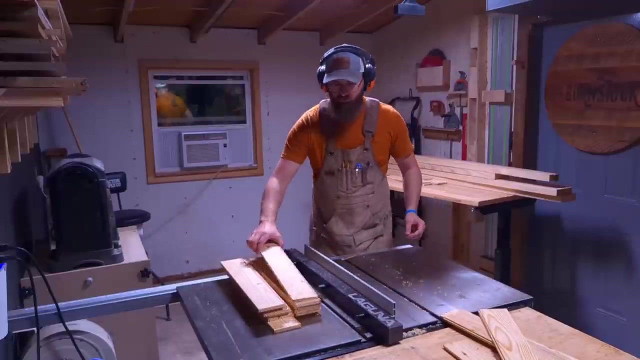 angle And then, once you get to the end, you can do like a cope cut. You'll see here where I'll shimmy it back and forth to take out that little bit that's left And that'll also smooth out all the grooves that are left. by using the Diablo blade, It cuts in a like a v-groove, So you make 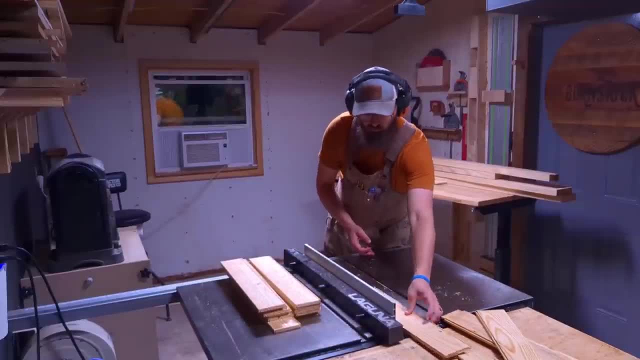 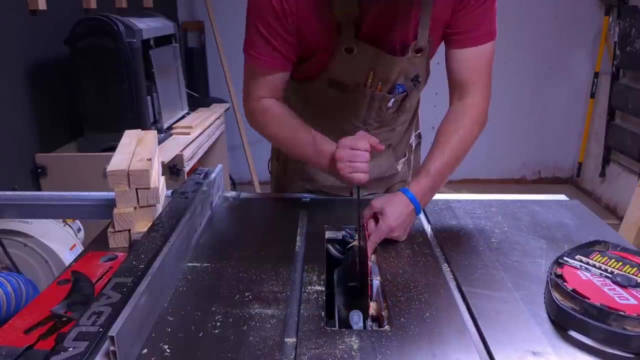 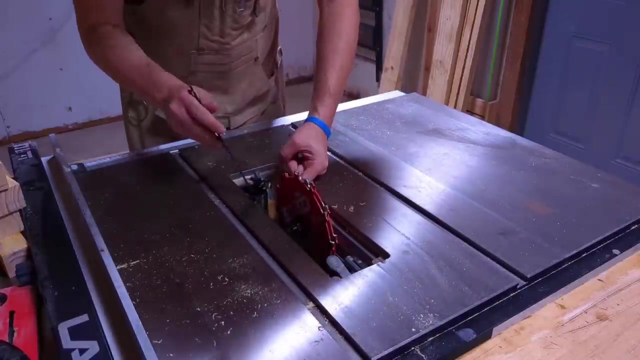 that nice, smooth and flat. It takes a little bit of time, It's easier with a dado stack, but it can be done without a dado stack. That being said, say hello to my dado stack. So I've had a dado stack for a few years now And it is a very handy tool to have if you can afford to put one in your 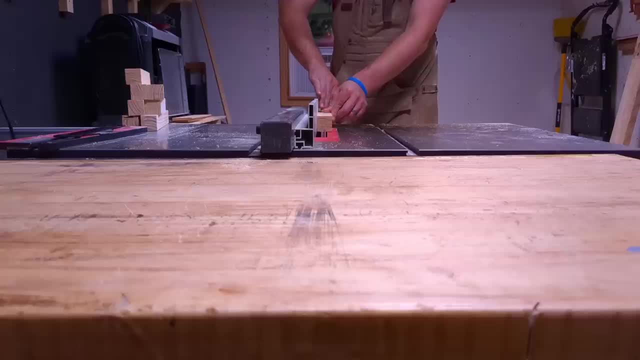 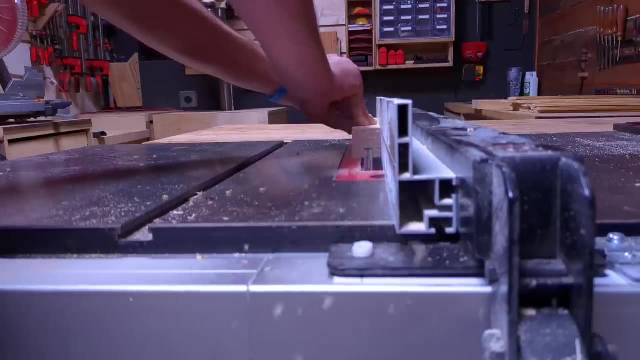 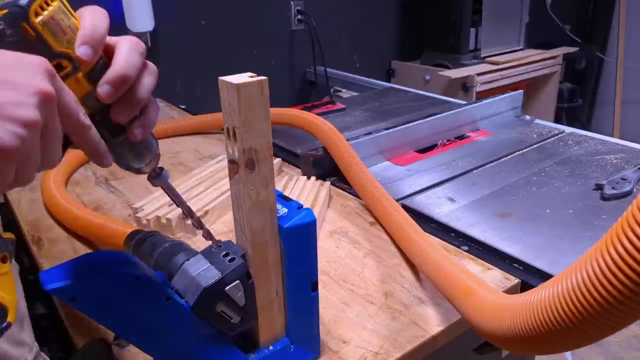 shop. Right now I'm using the dado stack to cut out the groove for my aprons that's going to house the shiplap. So this groove is about seven, sixteenth inches wide by a half inch deep, And you should. I didn't do it here, but you should try to get those to be the same width. 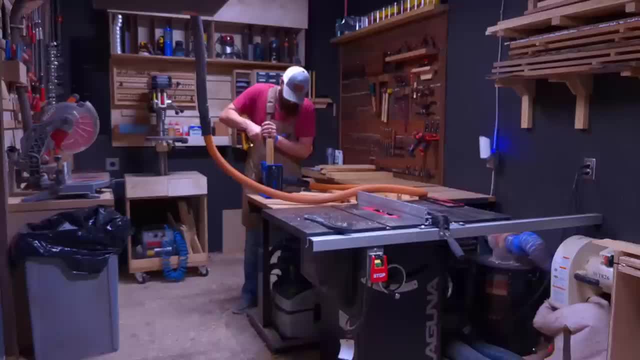 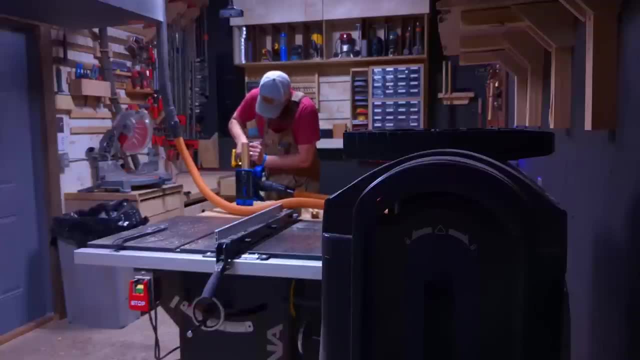 The outside edges. those should be the same width. But again, I wasn't paying much attention to what I was actually doing. I was paying more attention to the camera. I'll do better next time, but it still doesn't mess up the project. Okay, so with almost everything cut out, we're going to start. 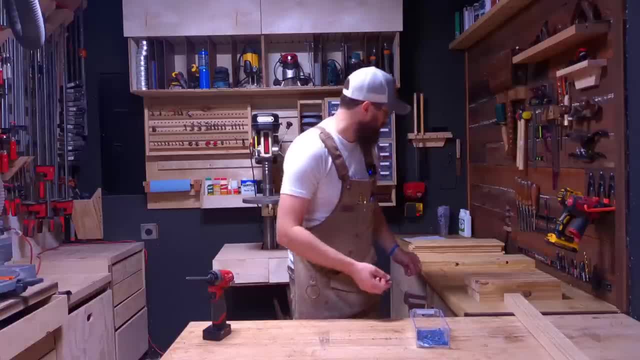 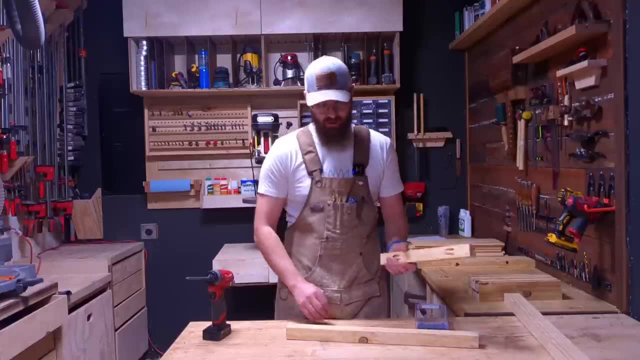 with the assembly And I'm going to kind of run through the assembly pretty quickly. The instructions should be pretty detailed on how to do it. It's very simple: Once you get the first step and second step, you just repeat the process. So we're going to take our aprons and our legs. I'm 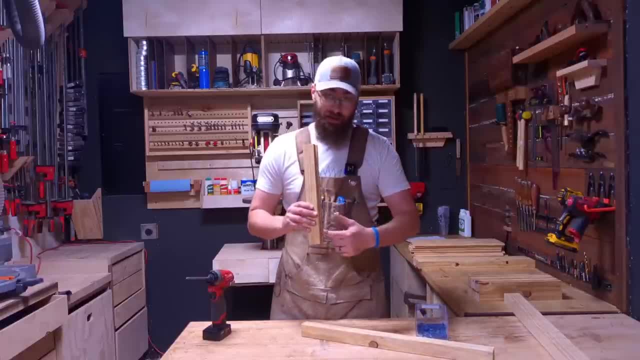 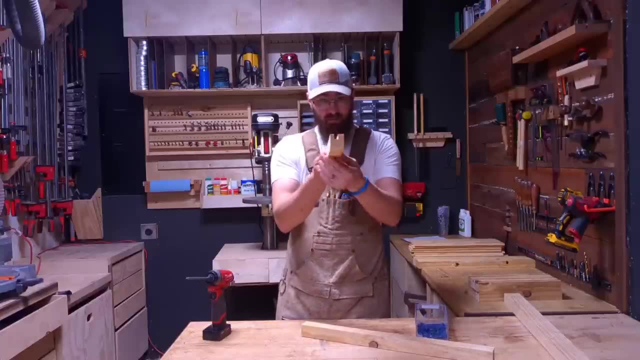 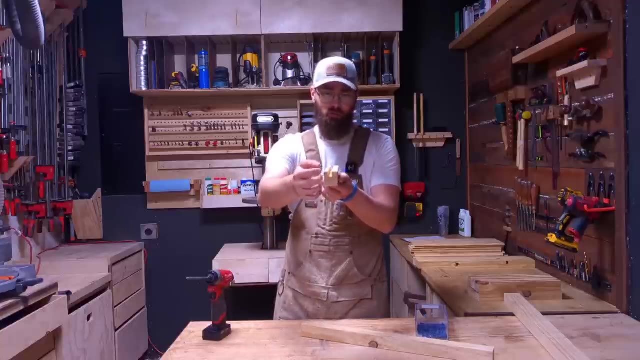 going to connect the first apron with the dado facing down. I miscut this So I miss. I actually messed up the layout on the dado, which is fine. If you do this, you want the thicker side stick into the inside of the planter box. I want to put this thinner side, which about a half inch- 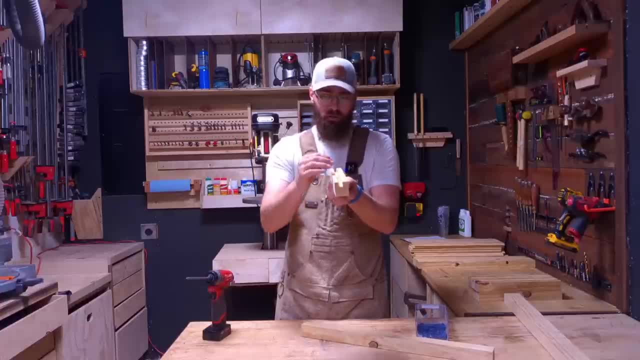 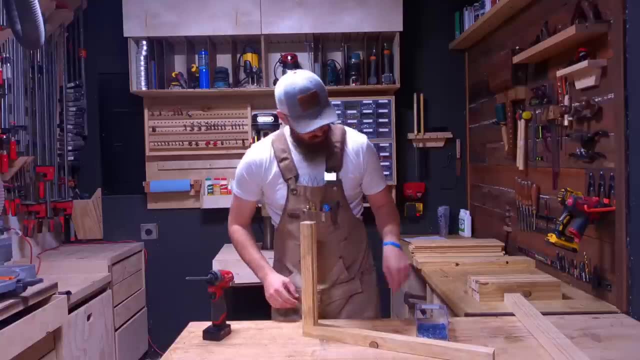 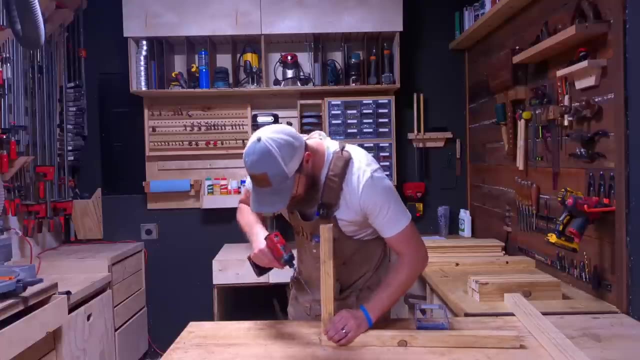 thick lip and we'll put that to the outside of the planter box. I'm going to put the thicker side inside and that's so that it will support the actual planter box bottom. So all we're doing is taking the Kreg jig, connecting it to the top side of the leg You want to make. 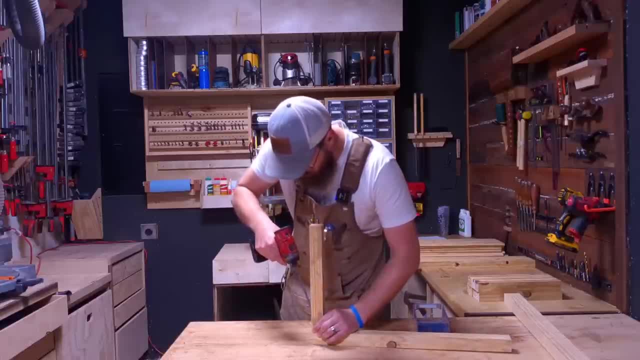 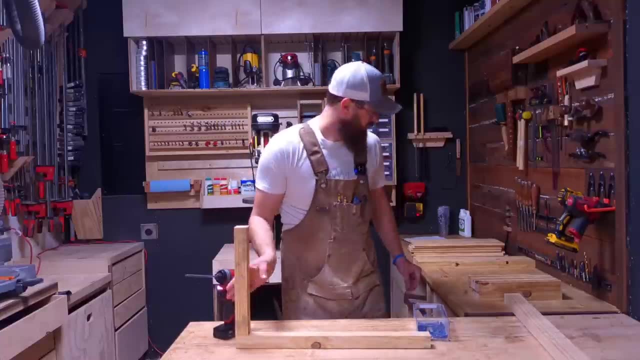 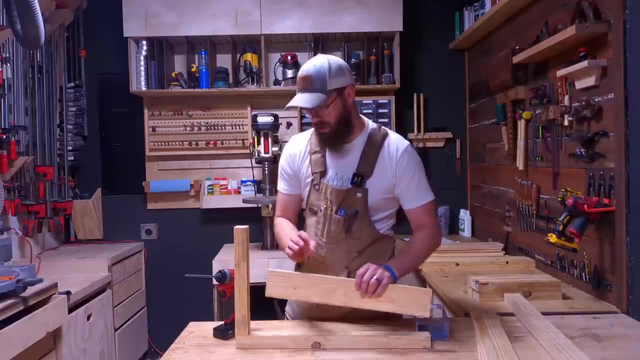 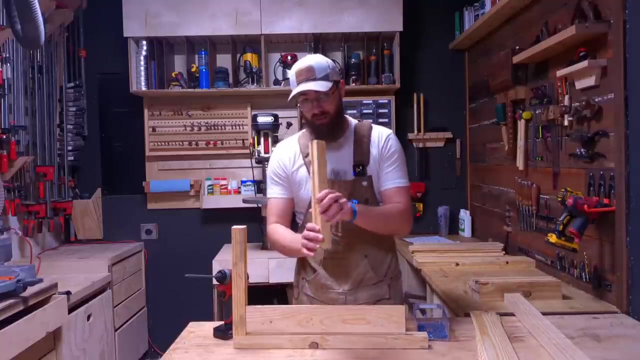 sure this is flush and screw it down. Then I'm going to take four pieces of my shiplap and this will give me the layout for where the bottom is. It doesn't have to be too complicated, just simple, simple, simple. Make sure you have the same thing on the outside. 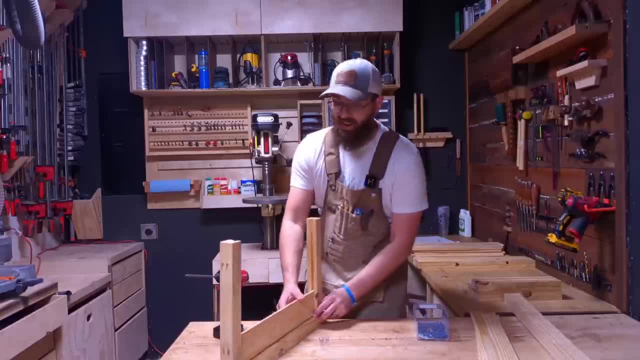 the thickest part facing to the inside. If you mis-cut it like I did, I'm going to have to do it again. If you mis-cut it like I did, I'm going to have to do it again. If you mis-cut it like I did. 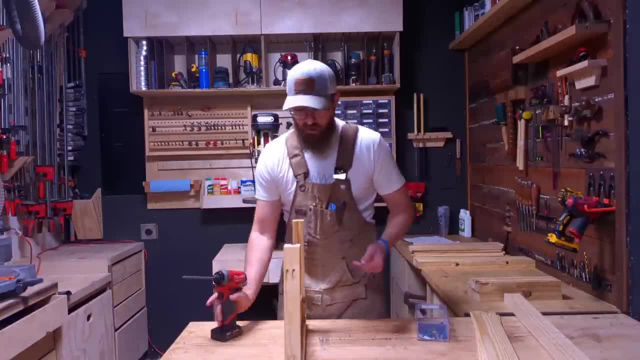 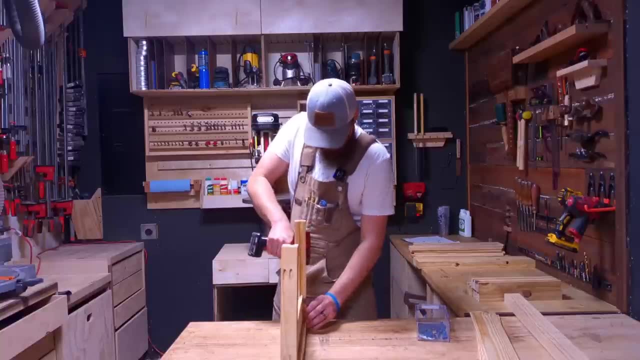 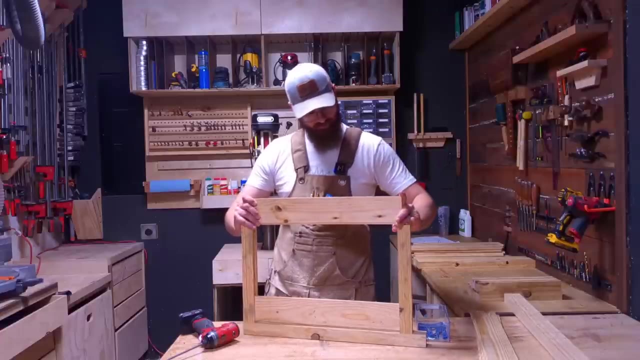 I'm going to have to do it again If you mis-cut it like I did. I actually made a few mistakes on this one, but it's still going to work out. So now I can take my shiplap and put it in there And the reason that I did shiplap. 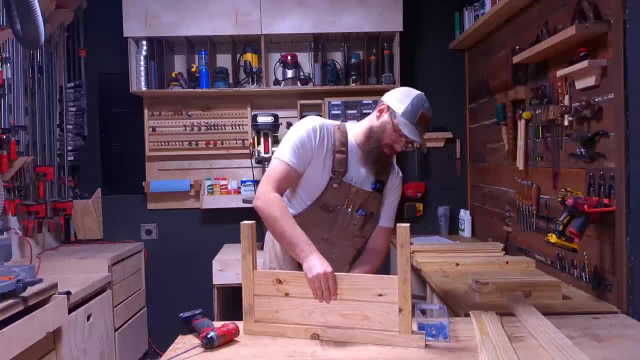 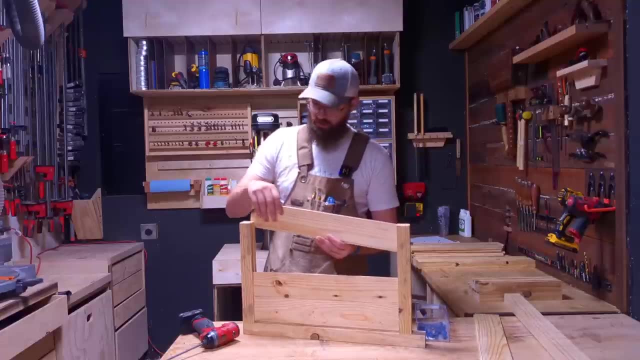 rather than gluing a panel is because I don't want the panel to split. This wood has a lot of moisture as it is Being exposed to the elements, it's going to expand and contract and it's already doing a lot of that, as it is like I said. But being in the 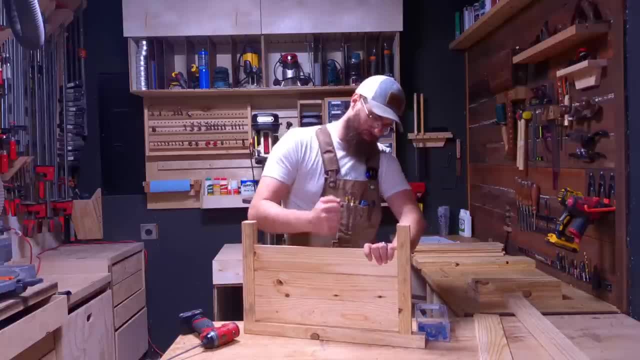 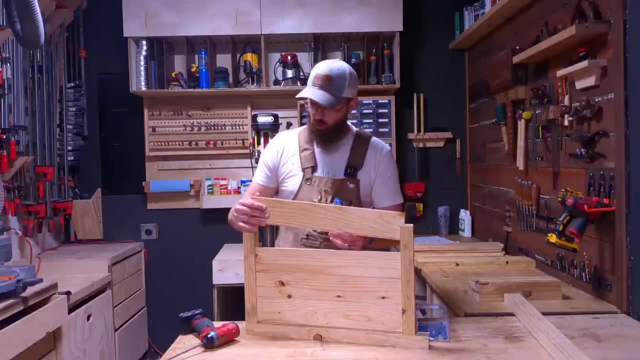 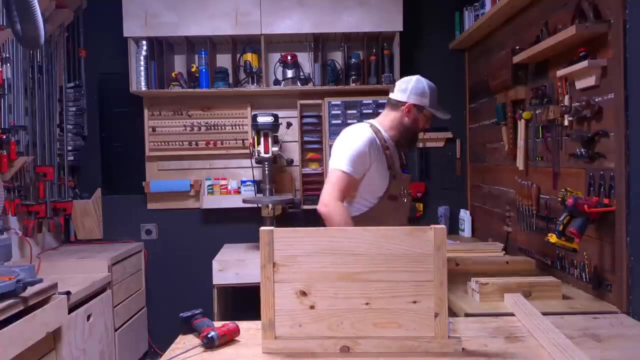 elements. it's going to do it even more and then panels will split With the shiplap. I have some overlap that whenever they kind of expand and contract, there's still going to be no gap, no holes, And that's it. We're going to take our next leg and attach it like so. 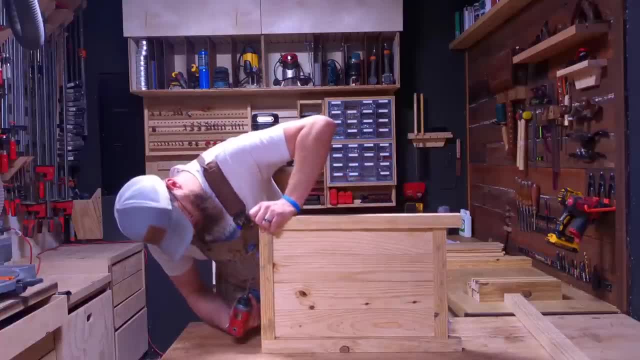 And that's it. We're going to take our next leg and attach it like so, And that's it. We're going to take our next leg and attach it like so: If you don't want to use Kreg Jig, you could do dowels or something like that. 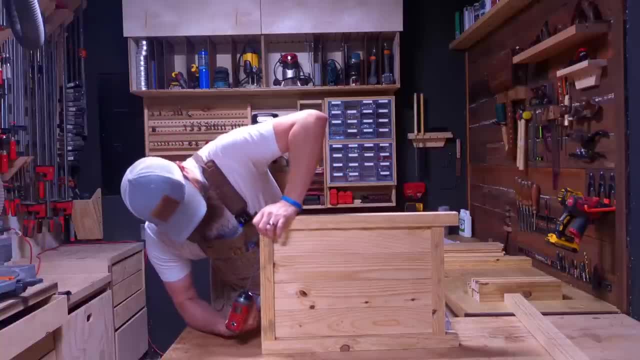 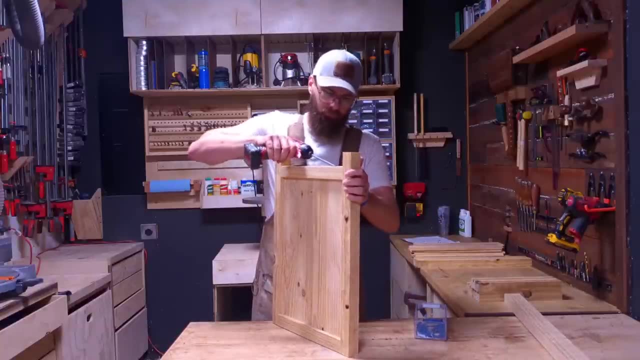 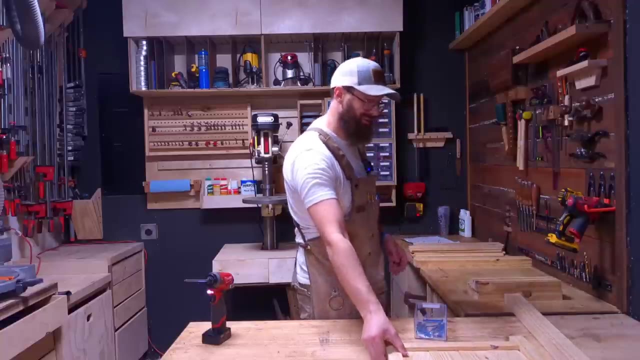 I have no issues with using Kreg Jig for something like this. So that's the first panel. We're going to make the second panel, then we're going to connect the two. You're pretty much going to repeat the same steps, so I'm not going to spend a lot of. 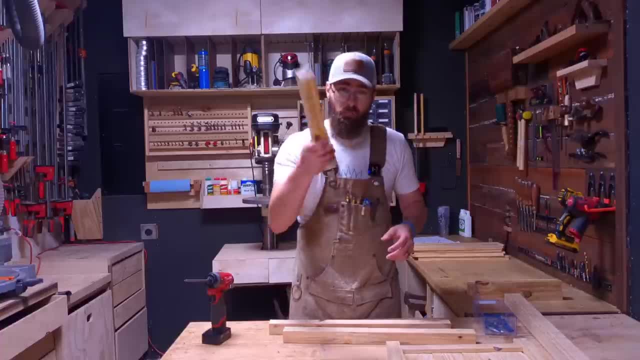 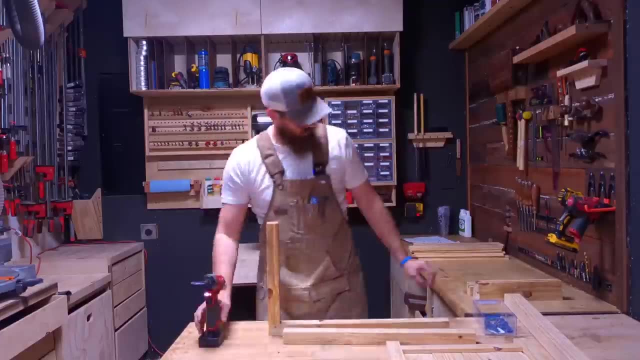 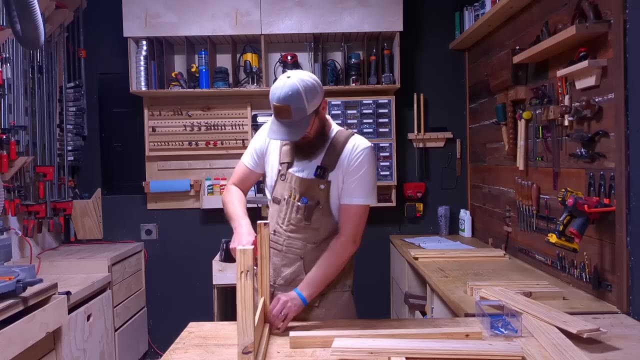 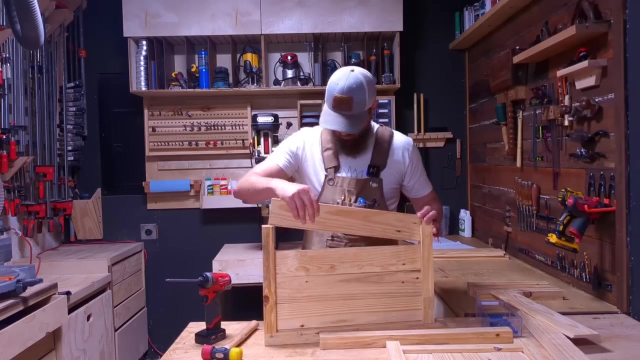 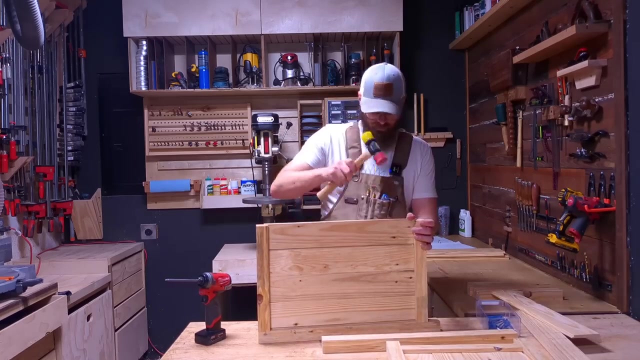 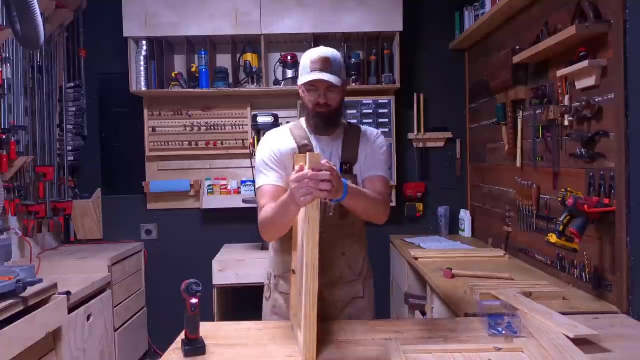 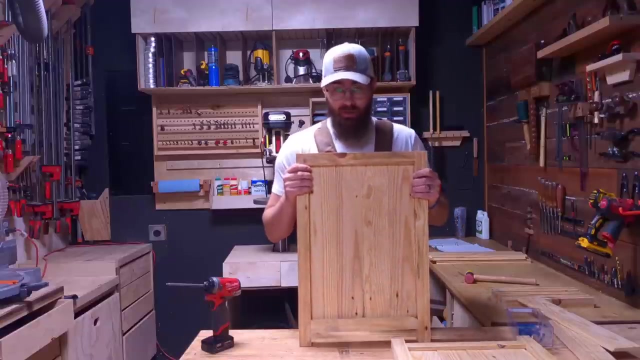 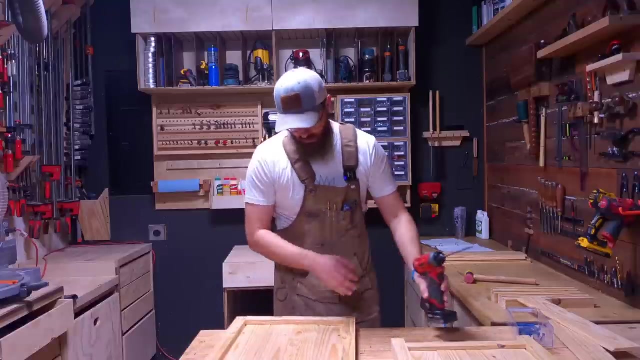 time talking about it. I'm just going to do it and speed up the recording. You want to be mindful that you don't close yourself in on a box before putting in your paneling. A way to avoid that is: I want to take one of the panels and I'm going to do one runner. 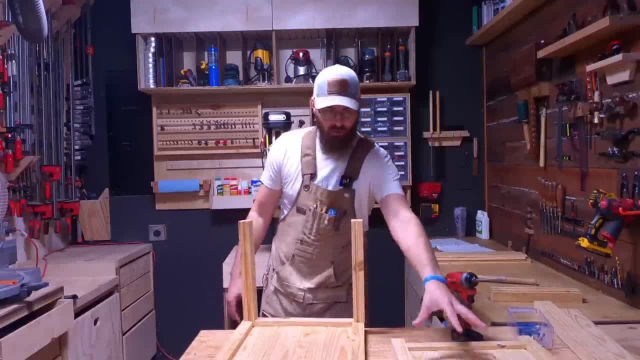 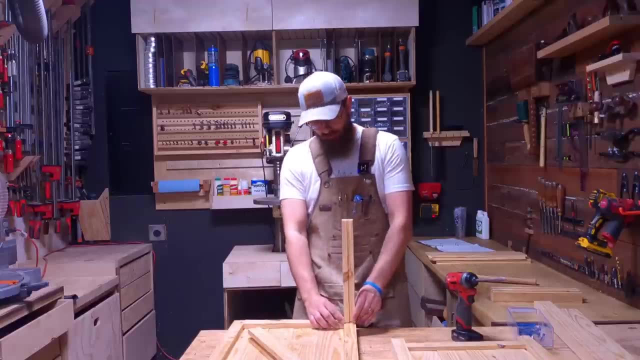 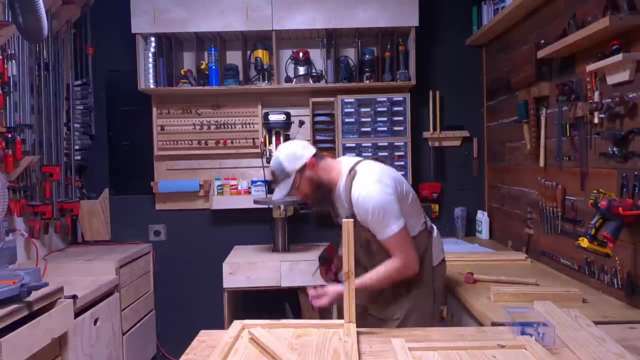 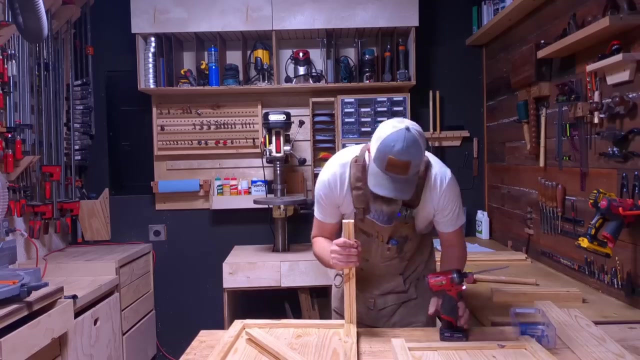 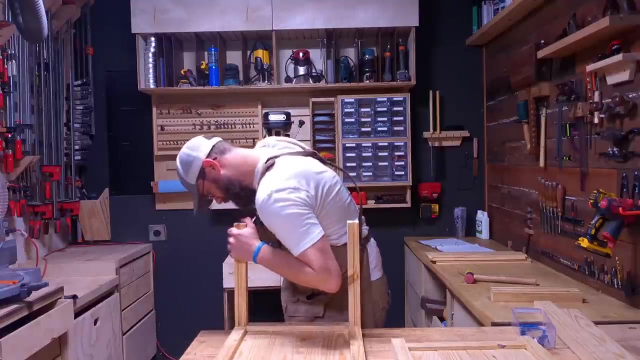 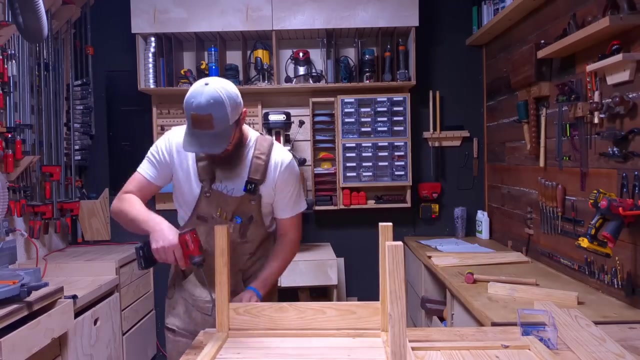 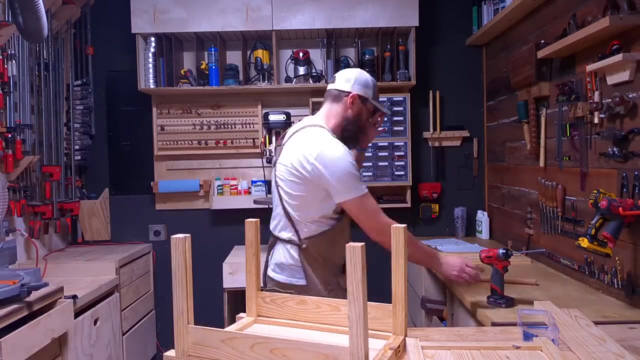 on each side, place my shiplap, do the bottom runners And then I'm going to use this other panel to cap it- Cat-like reflexes. I'm sitting here doing woodwork and I should be doing parkour, So in the middle I just leave it like that. 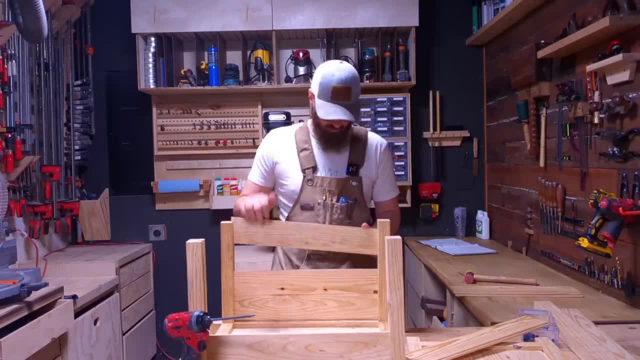 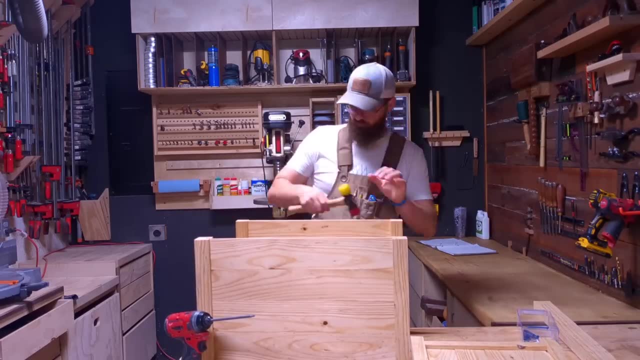 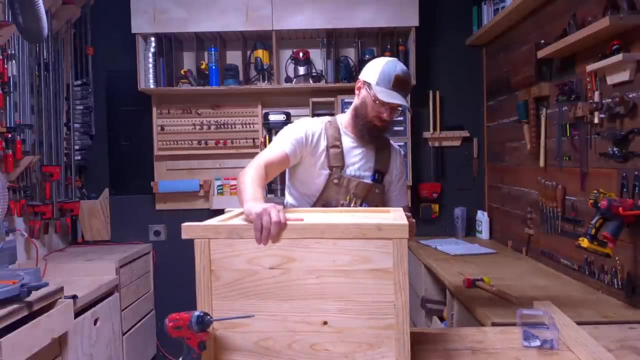 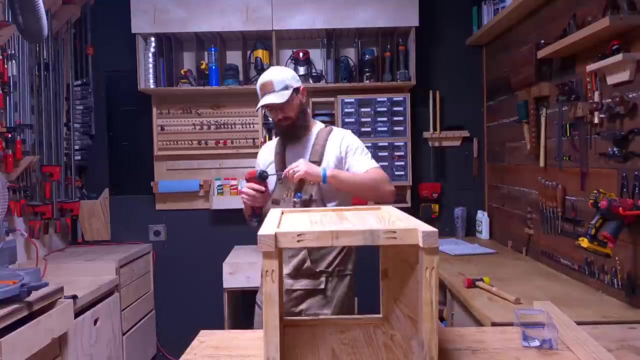 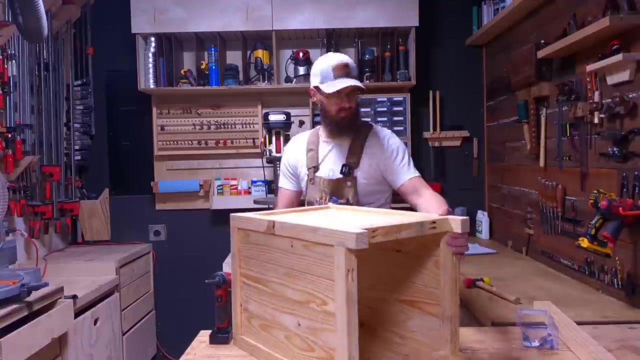 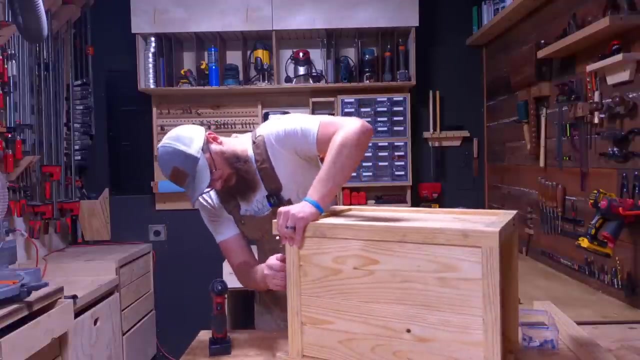 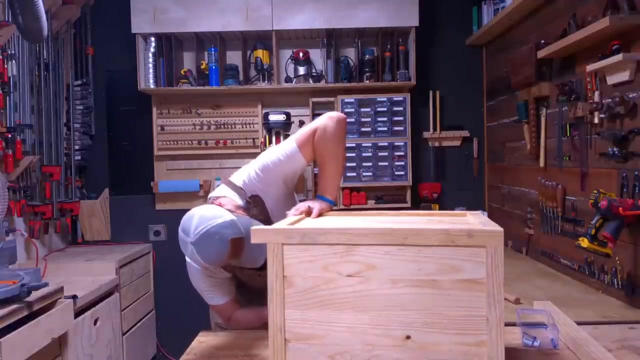 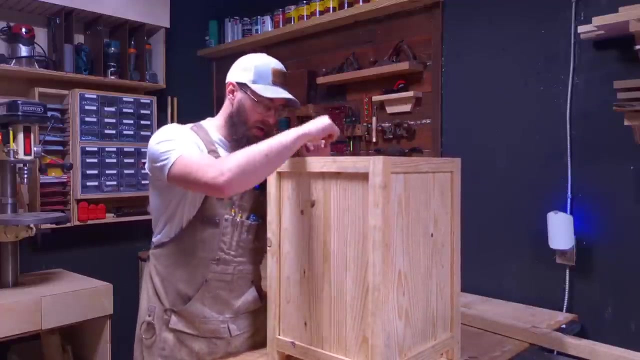 I'm not doing a lot of work, though. I'm doing just a little work, And then you can just get your thing done. OK, Alright, Perfect, All right. So that is the box. All we have left to do is the trim on the sides, and we'll do a cap in the bottom and that will finish the box. 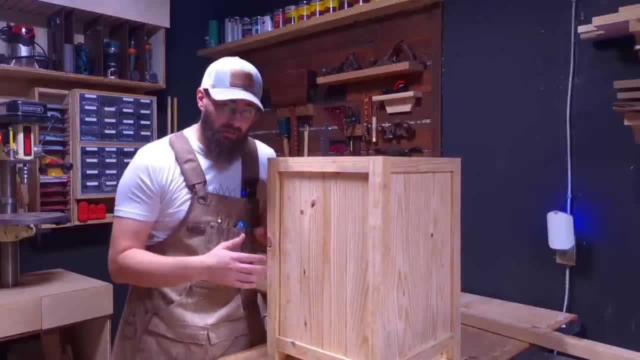 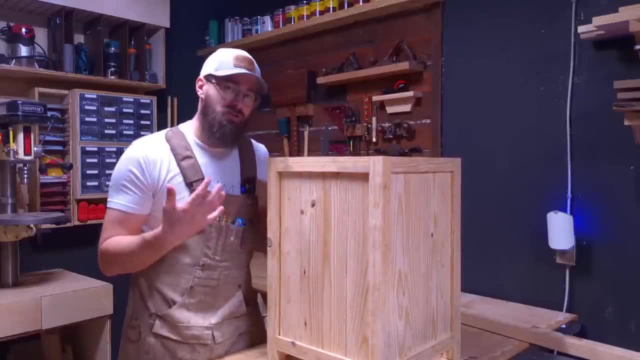 But first I want to make the cap. We're going to use whatever's left of the 2x6s to make the trim and to make the base for that, because they don't have to be really consistent pieces. We can kind of just use what we have left over. 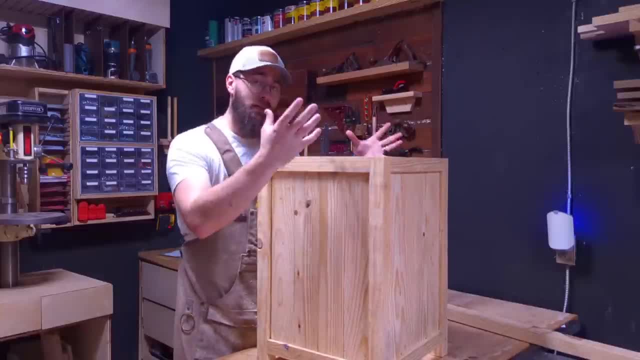 So we're going to make the cap, then we're going to put the box to the side and we're going to make the obelisk to go on top. So our cap is going to be 2 1⁄4.. 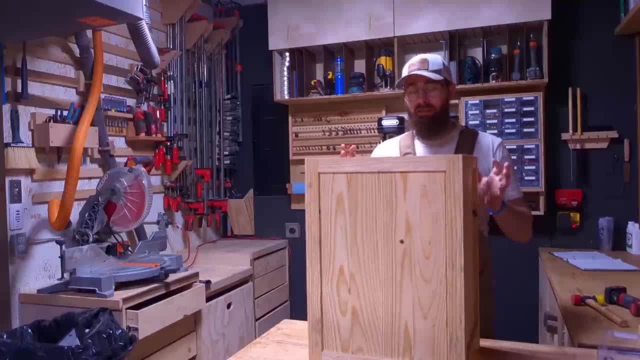 Now, if you followed exactly the way that I have the plans laid out, it should work out just fine. to where you cut those: to inside angle. to inside angle is 13 1⁄2 inches. However, I kind of messed up on my shiplap and I went a little bit too far in. 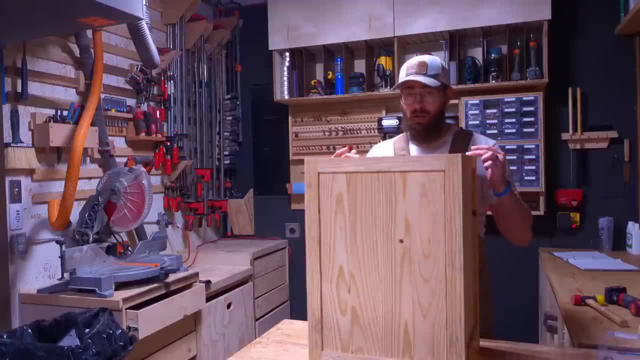 Rather than an eighth of an inch, I did a quarter of an inch, So now I have 13 1⁄4 runners. That's fine. I'm just going to make my cap 13 1⁄4 long, from inside angle to inside angle. 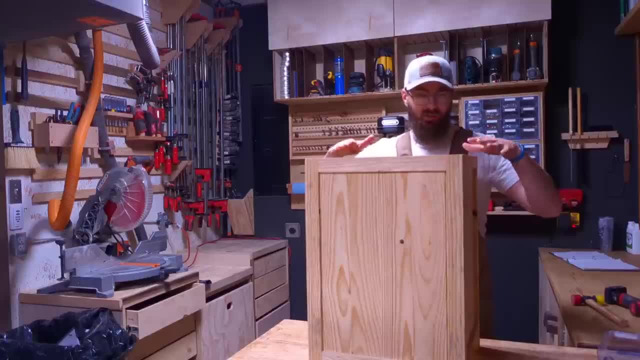 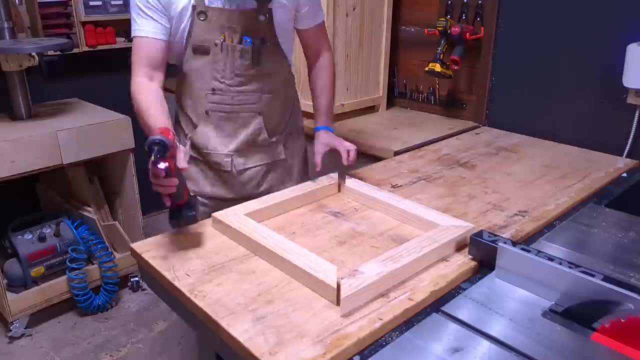 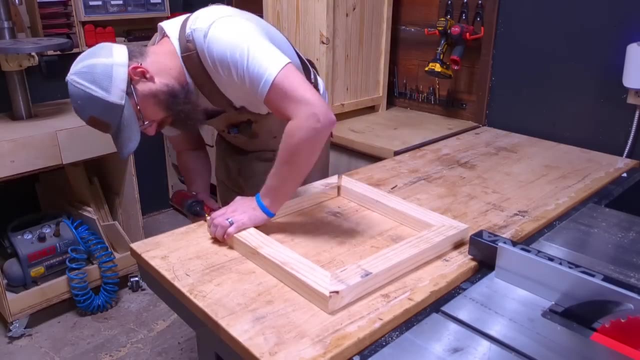 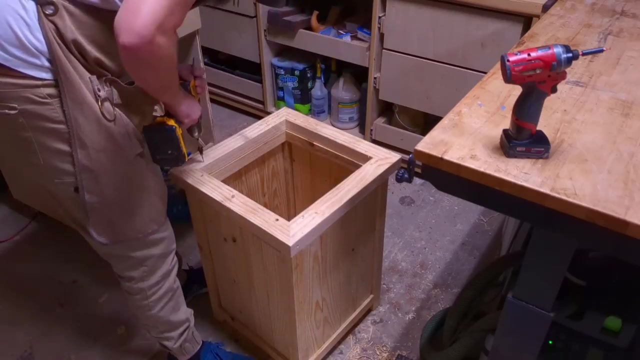 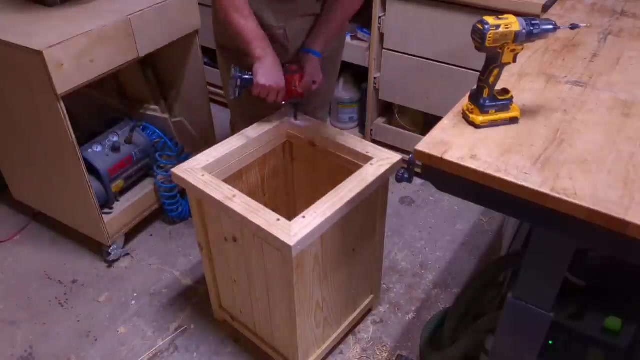 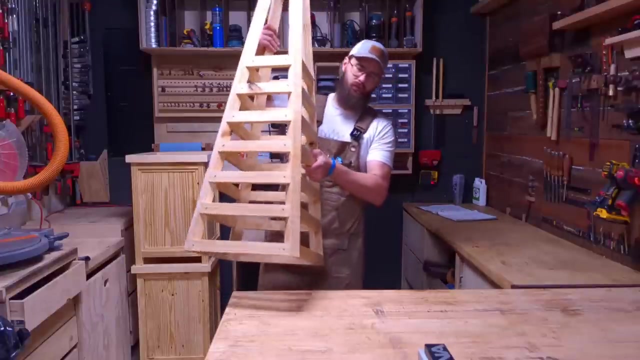 The outside angles will still meet up. It'll still cover what I need it to cover. It's really just for decoration and to give the obelisk something solid to sit on. All right, Let's talk obelisk. So this obelisk is pretty simple to do and there's a jig that we're going to do to make it even more simpler. 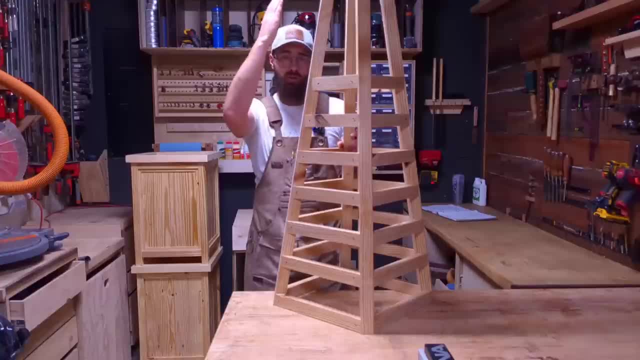 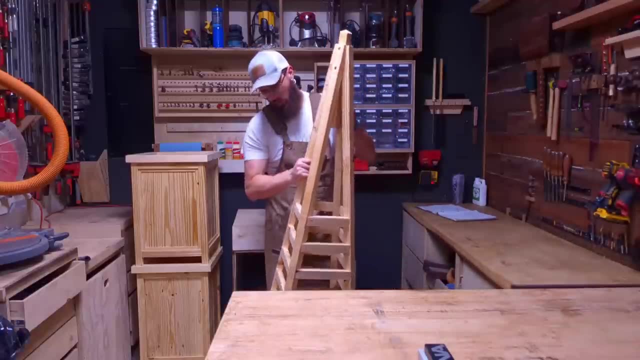 The bottoms of the legs are cut at 10-degree angles. The tops are also cut at 10-degree or 80-degree tapers. It depends on which reference you have for the angle. I'm going to show you a jig that's going to make it really simple. 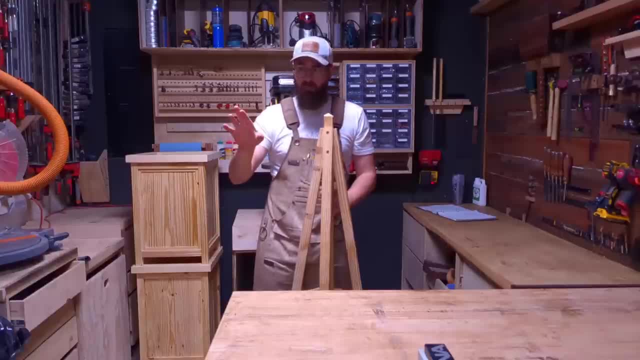 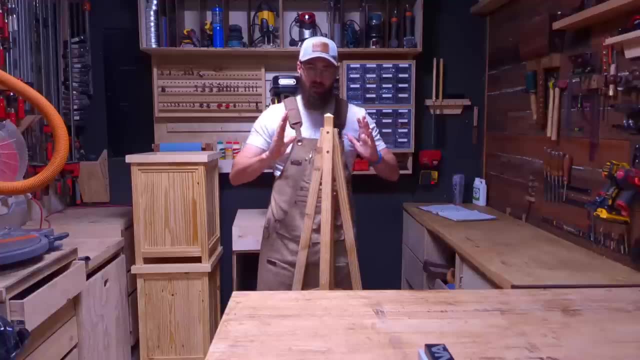 The first thing I want to do is put a 10-degree cut on the bottom of my remaining 1 1⁄2 inches. Then I'm going to build a jig that will cut this taper right here for the top so they all meet up at a nice flush surface to this center post. 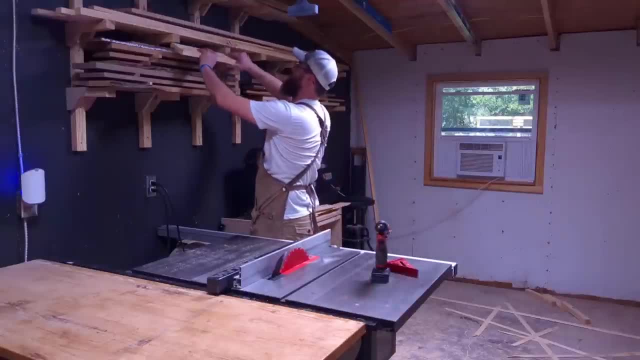 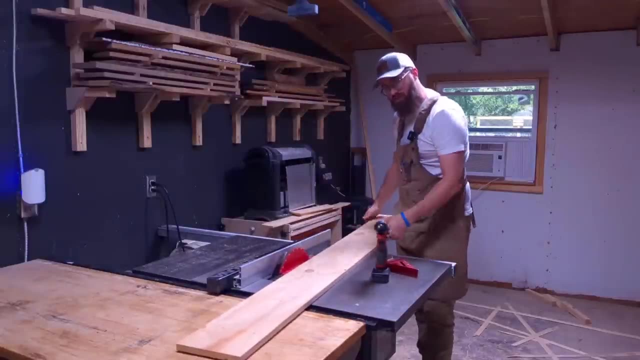 Okay, So to do the jig for the legs, we're going to use some scrap wood. I have a long piece of plywood. You can tell I've already made the jig. I'm going to flip it over and start from scratch. 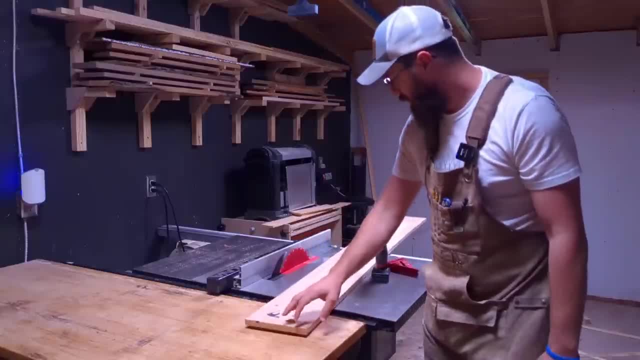 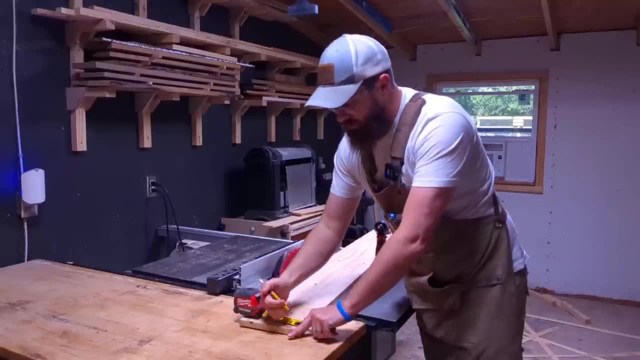 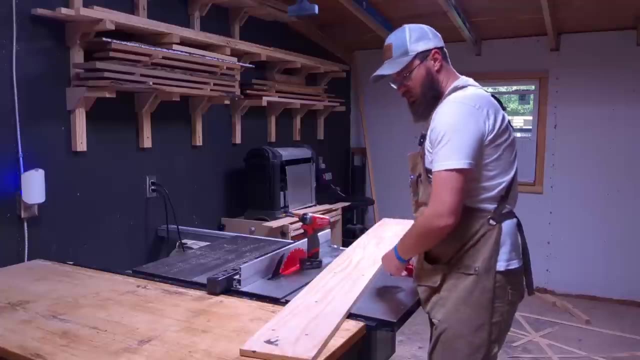 So this is where I want to cut my taper. on this end, I'm going to make me a mark at about a 1⁄2 inch, because that's what I want the top of my taper to be. Take your square, Make you a line. 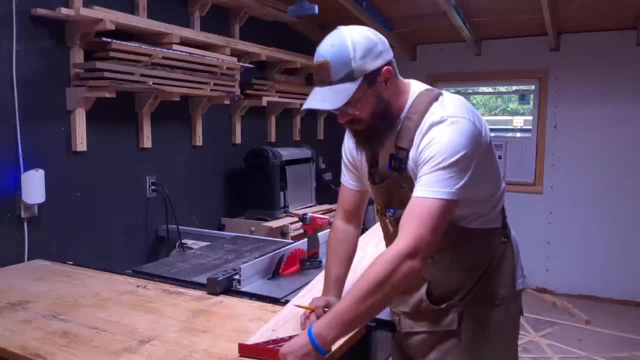 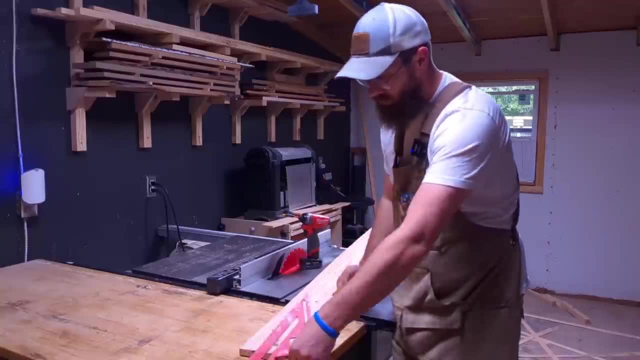 All right, Now we have our straight line. Set it on that line. I'm going to pull this back to 10 degrees. I want to make my line Now. I'm going to put it back. I'm going to put my backer on that 10-degree mark. 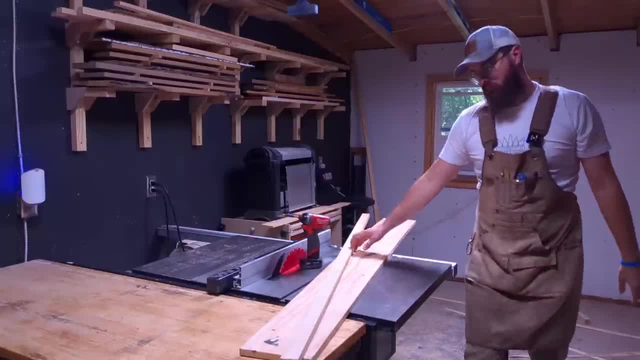 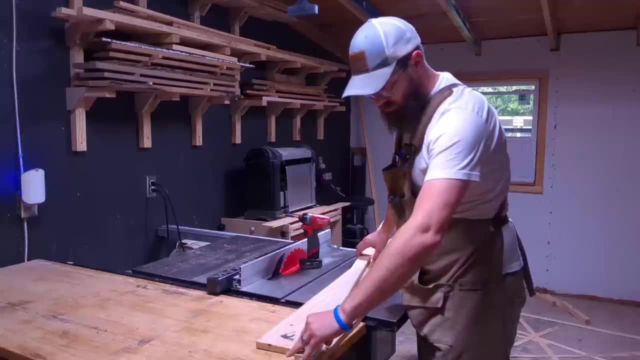 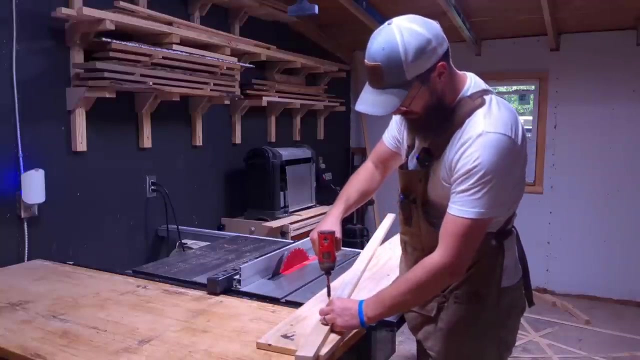 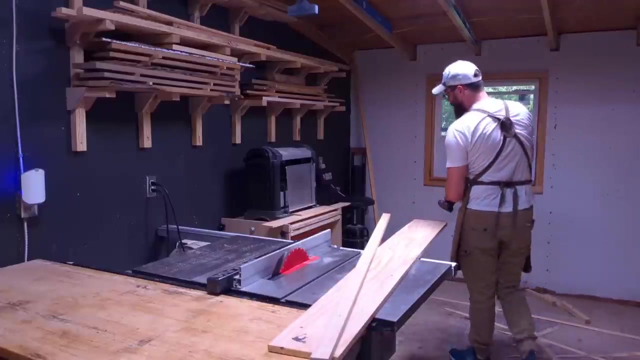 All right. So I'm going to put my backer in place, We're going to set it on that 10-degree mark And we're going to screw it down, And that's it. There we go. So now all I've got to do is set the fence. 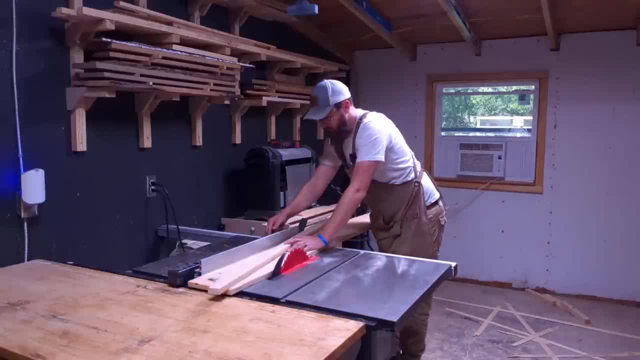 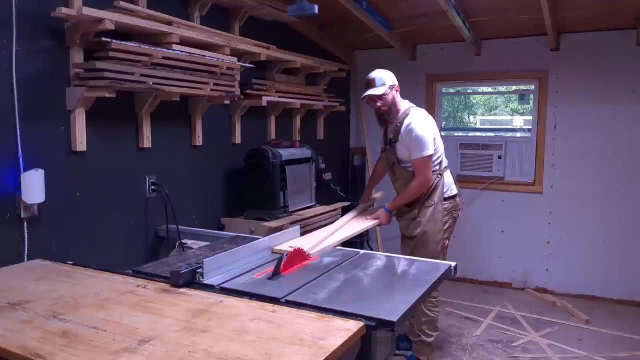 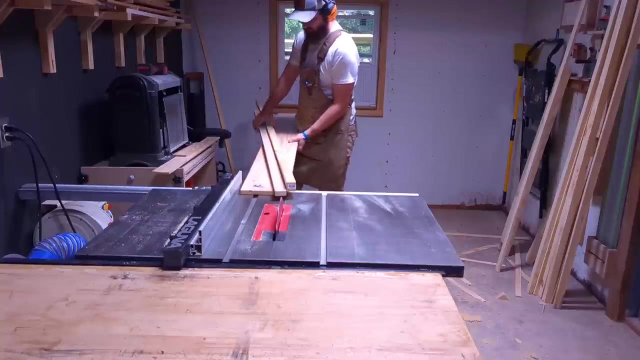 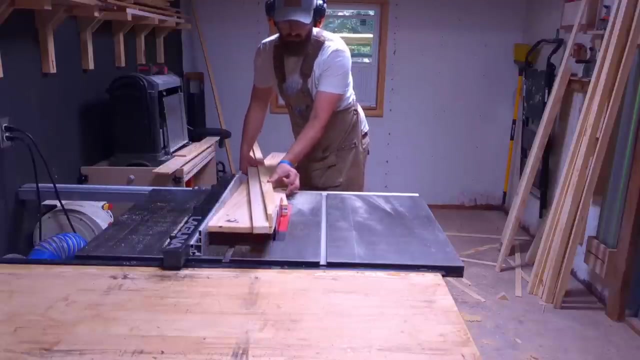 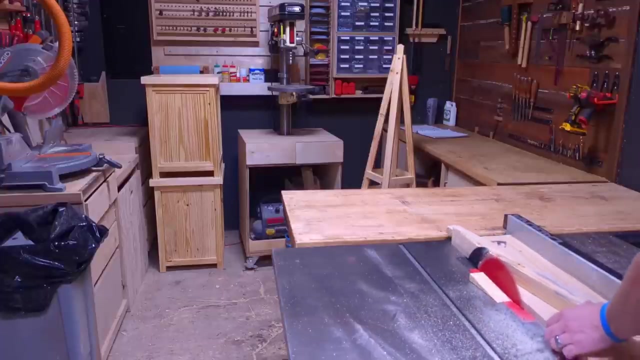 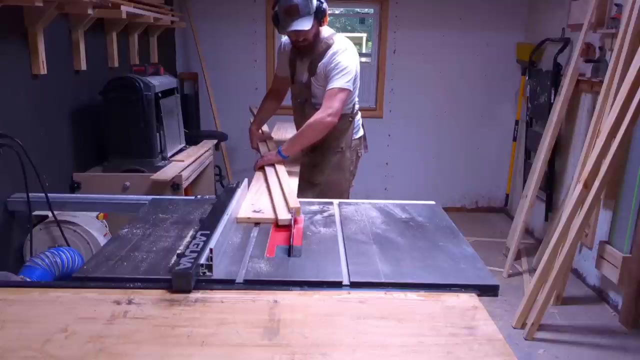 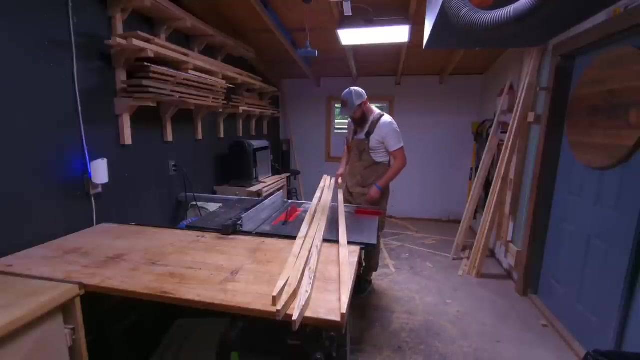 to where it's the same width of this plywood. I want to put my leg on there and I'm going to run it through, get my taper and move on to the next one. All right, Okay, So with our tapers cut, very, very simple, very easy. 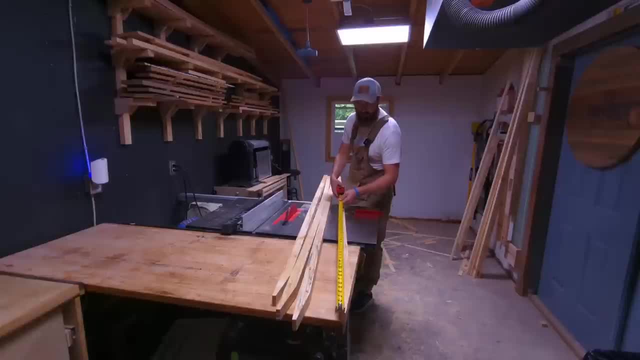 Even with filming and recording it took less than 10 minutes, if even that. Our legs are going to be 57 1⁄2 inches tall. So I want to measure from the end of that taper the outside angle of the 10-degree angle at the bottom. 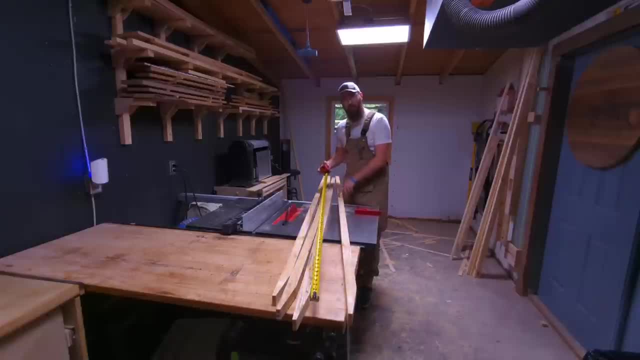 We'll measure from that end to the outside angle of the 10-degree angle. at the bottom It's 57 1⁄2 inches. So we're going to take it, pivot this back to 10 degrees and make our mark. 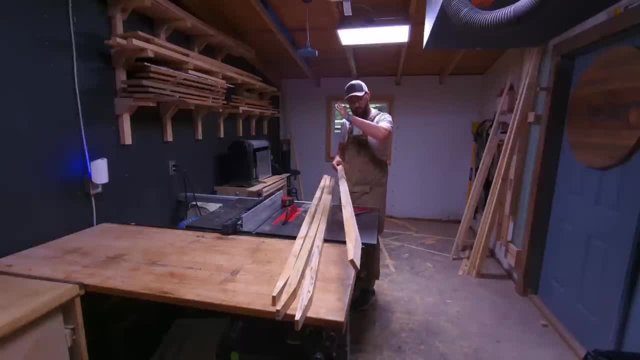 And so, once we cut this angle, what that 10 degrees is going to do is make the leg angle to the inside to meet that center post. Now, once I make this cut, I'm going to use this leg as reference for all the other legs. 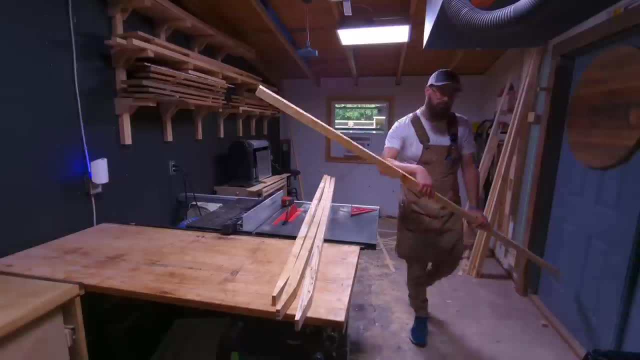 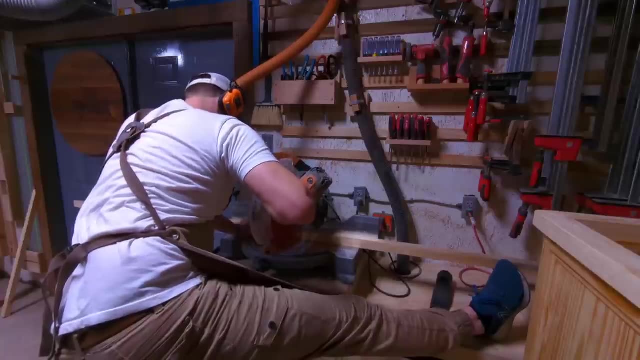 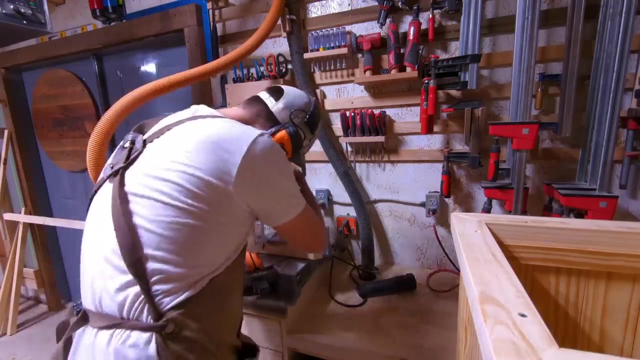 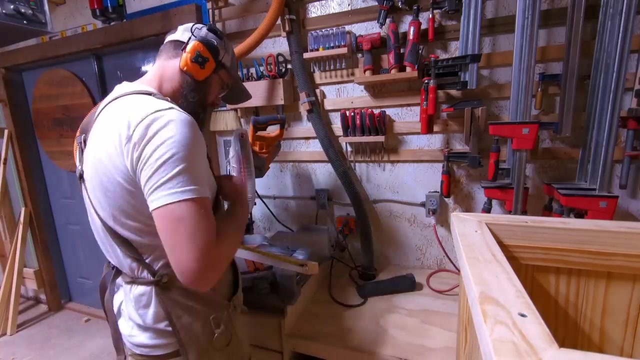 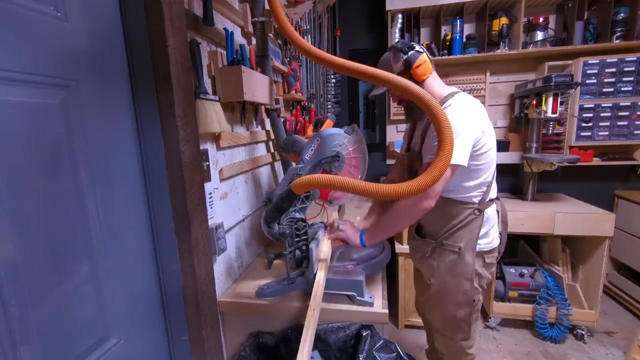 so that they're all the same length. All right, All right, So this is what it will look like. So this is what it'll look like. So these are the pitts Pen closer between sides. So this is what it'll look like. So these are the patterns. So let's go ahead and unfold our guide board. So let's cut around the idiom really right here. So these are the patterns. So so far writing in Japanese. I get that we look, looks like here. 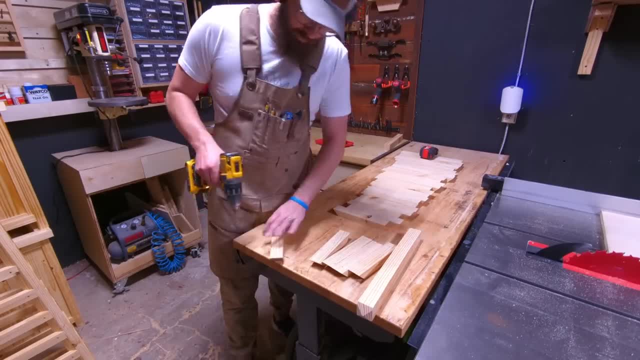 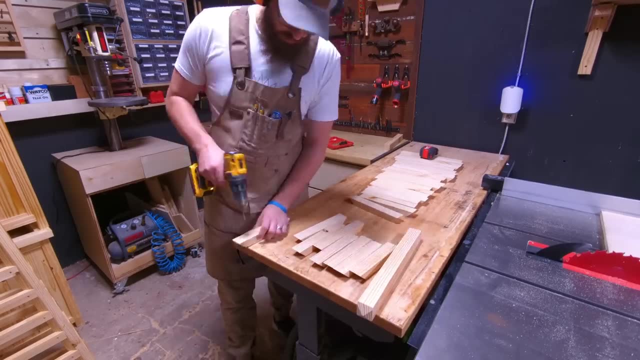 pieces that will make up the ladder for the obelisk. It is very beneficial to go ahead and pre-drill all of your holes for these instead of trying to pre-drill while you have it in place. It saves a lot more time if you pre-drill it before you try to screw it to the obelisk legs. 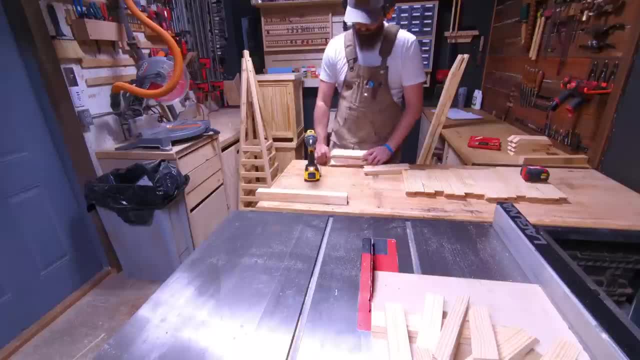 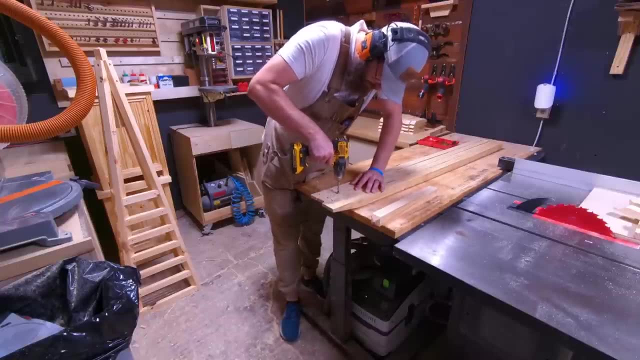 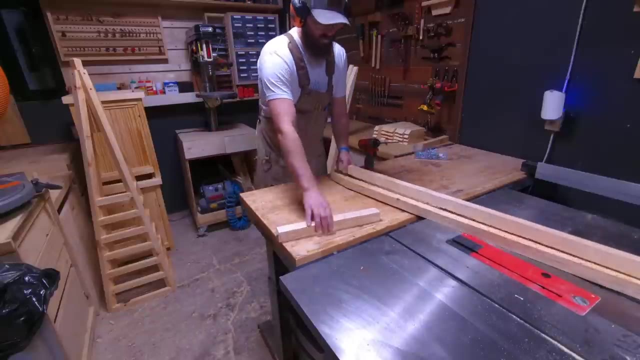 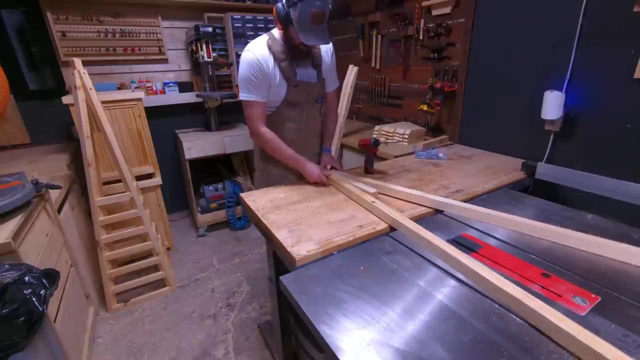 themselves. And right here I'm just doing a half inch by half inch hole just to give the screw head a recess. You can go back and put a dowel to seal these off. It's actually pretty advisable to do that so that you don't get water into those holes and it increases the rate of rot. And so here you. 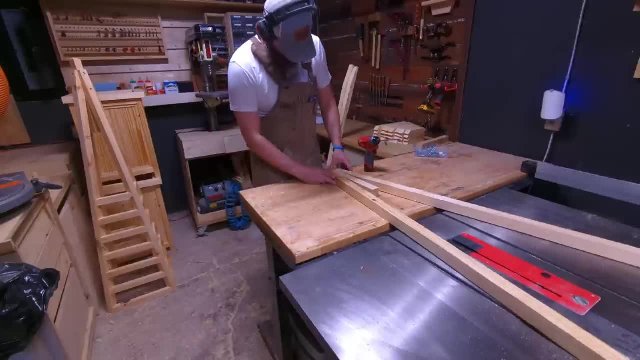 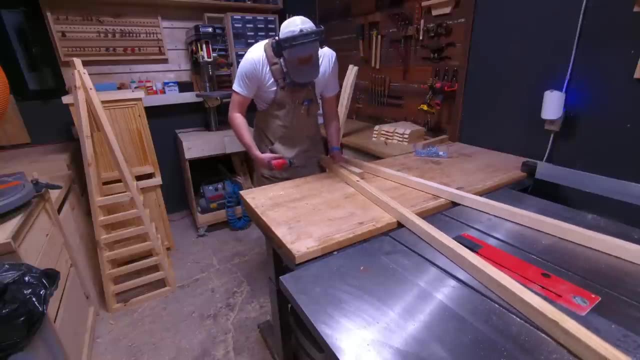 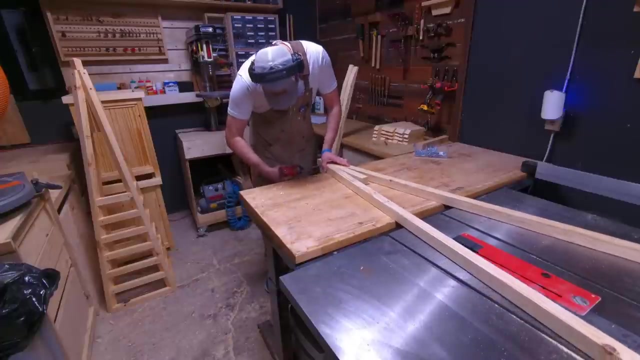 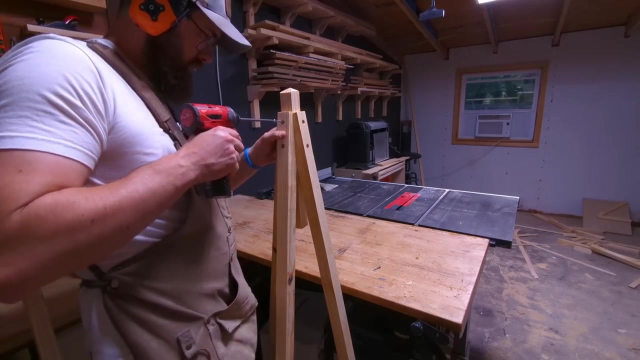 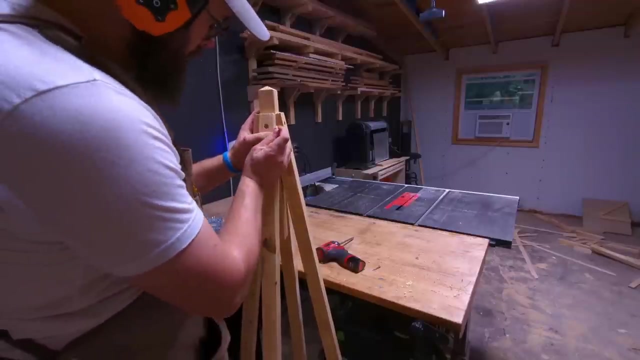 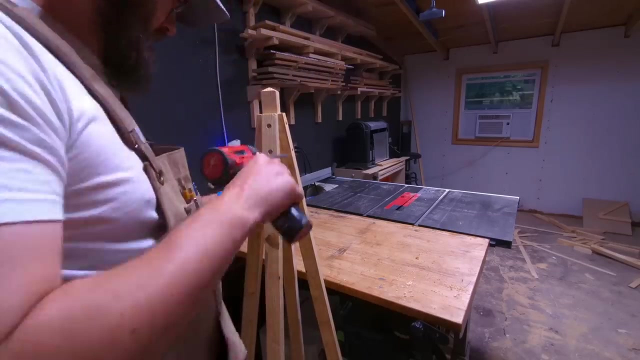 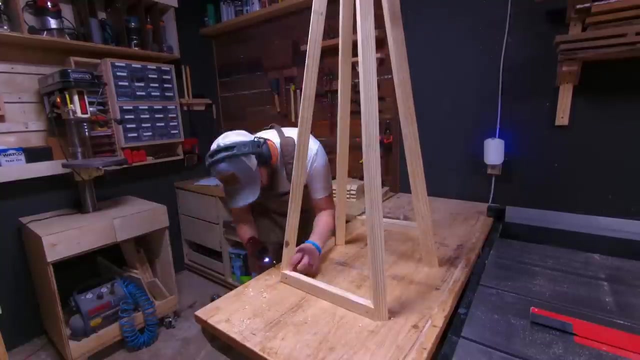 just lay it out as best as you can, using what you got. So I'm laying it out, I'm attaching the center post to two legs and I'm going to attach each leg on the outside later on, And so I found the easiest way to do this is do all of the pieces at the bottom first. 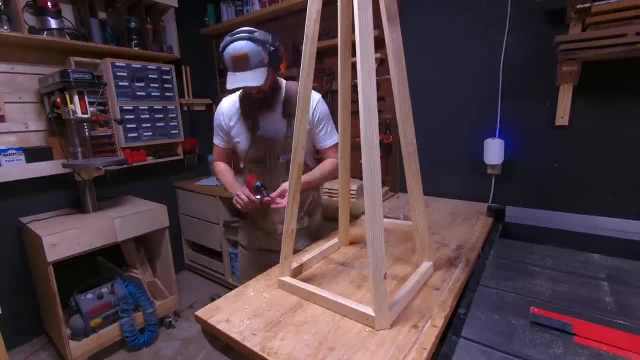 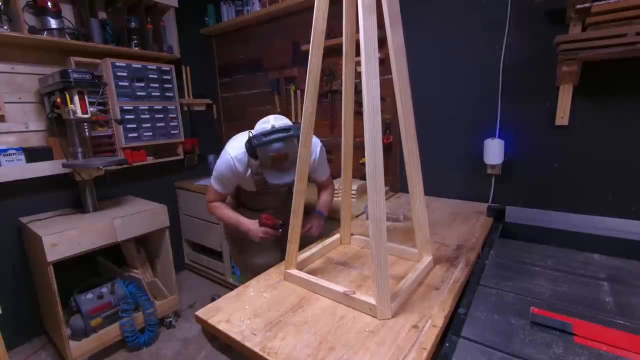 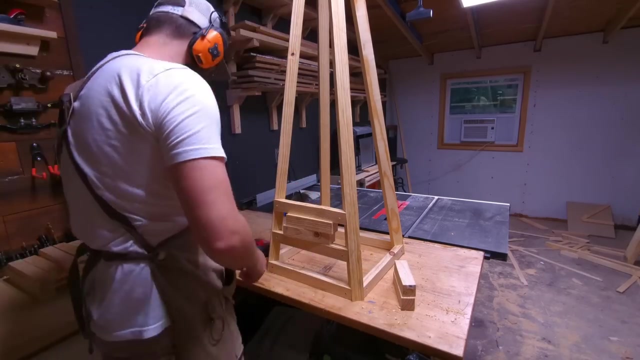 And then work your way up on each side. I took some one and a half by one and a half inch cutoffs that I had and I used those for spacers, which you'll see in a second. I used those for spacers to work my way up to the top. You just set your spacers on there, Set your ladder rung. 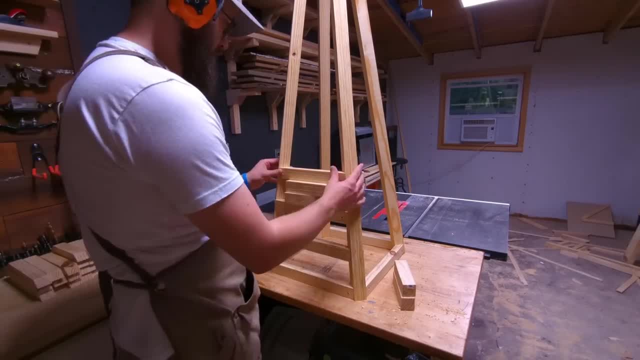 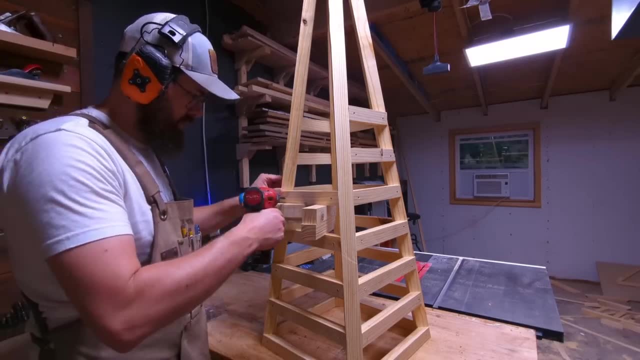 on top, Screw it in and move on to the next one. It makes the process so much simpler, rather than laying it out with a tape measure, And it makes it more consistent. Those spacers are going to be more consistent. The spacers are pretty much set. You're not going to mess up using a spacer. 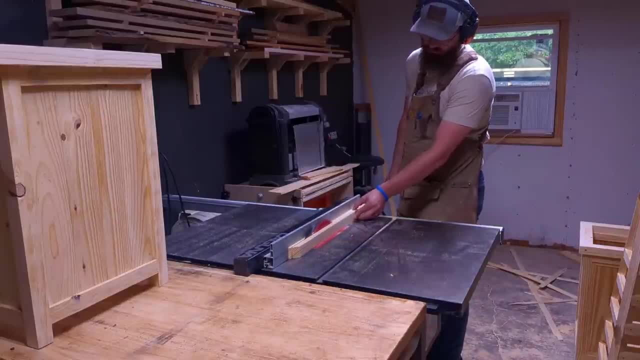 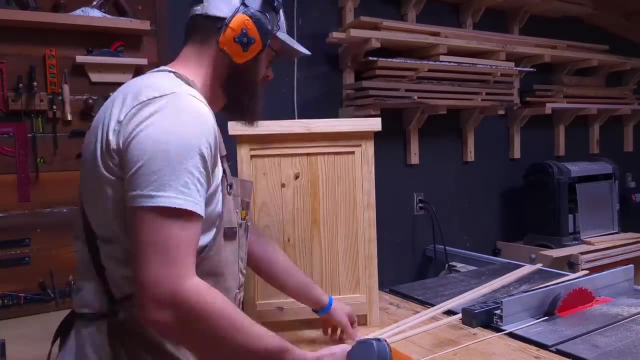 So, like I said earlier, the trim is just made out of the scrap that's left over. I'm cutting it a quarter inch wide by three quarter inches, I'm sorry, a quarter inch thick by three quarter inches wide, Laying it out in place, tacking it down. Simple, simple, You can make it as simple. 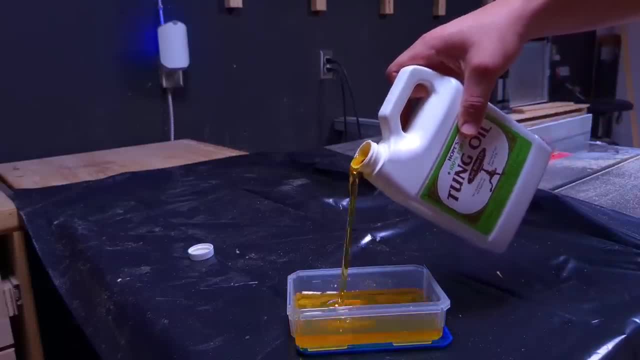 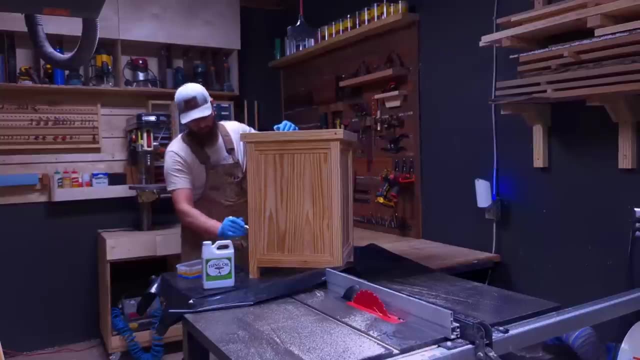 as you want Now this tongue oil. I will have a link in the description below. I'm going to have a link in the description. It is 100% pure tongue oil. There's no other chemicals mixed in with it. Tongue oil is a good exterior finish. You do want to put a couple of coats though It. 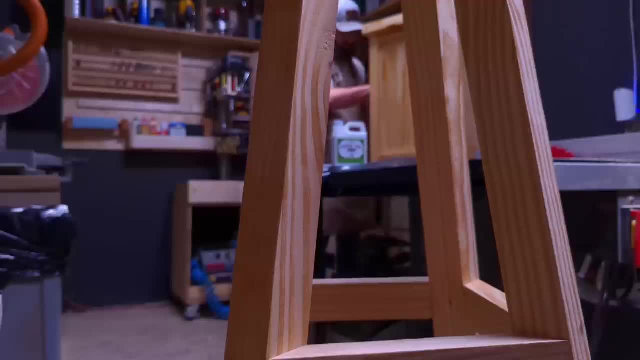 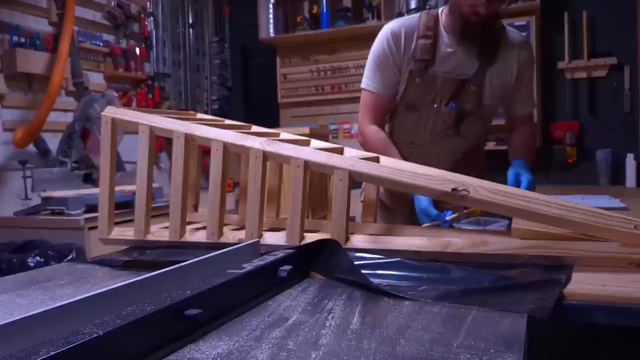 takes about a day for the wood to absorb the tongue oil. Then you come in and kind of etch it with a high grit sandpaper or even a scotch brite pad. Then you put your second coat. That's the base. I'll leave it open because when somebody puts a plant in this box it's going to be inside. 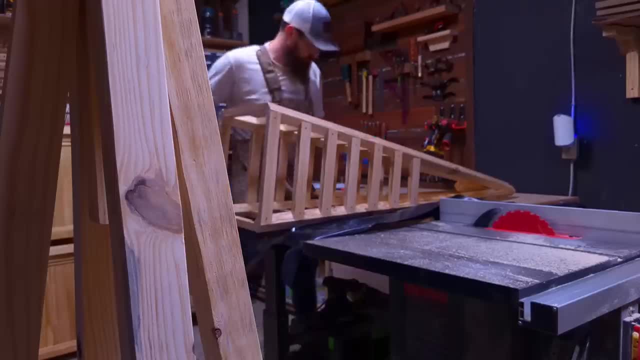 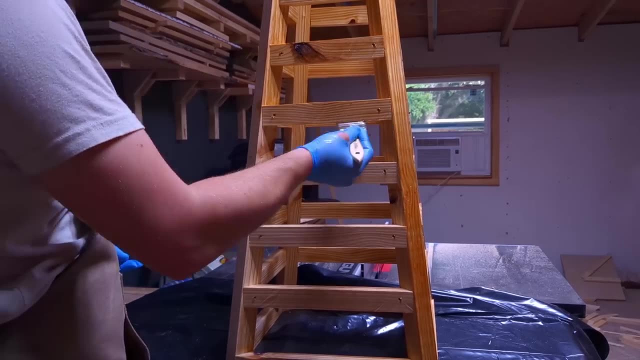 of one of the planter pots, So you don't need a solid base. They're not going to fill these up with dirt. Last thing: do not attach the obelisk to the box until you deliver, because they need to be able to put the plant. 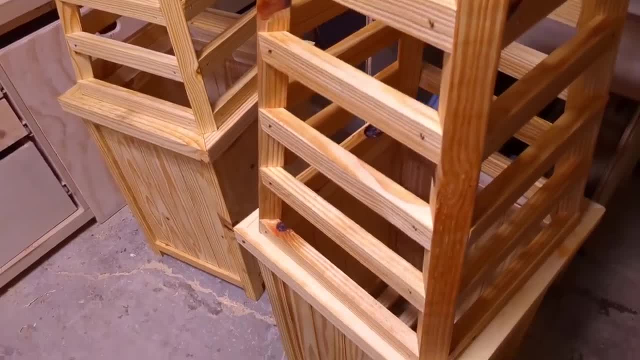 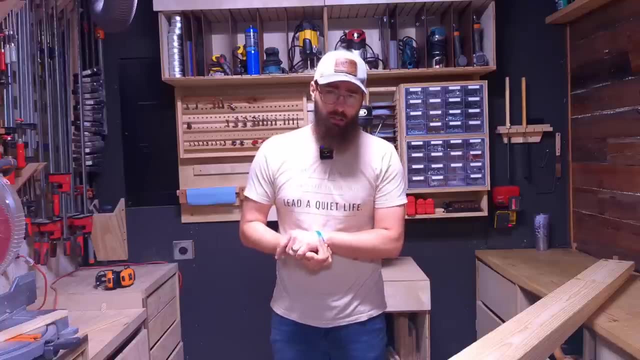 inside the box itself. So pre-drill the holes, give them some screws so that when they put the plant in, they can put the obelisk to the top themselves. Okay, so if you've stuck around this long, you probably found value in this video. You should like and subscribe. I'm all about. 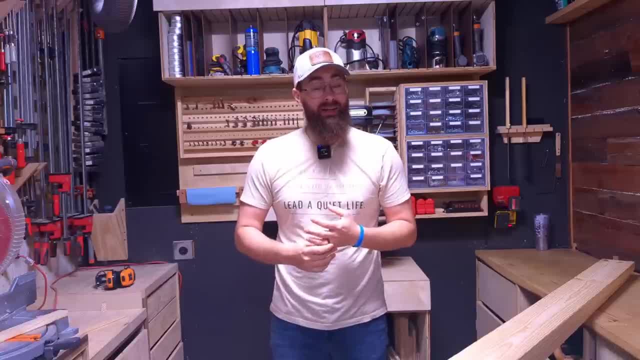 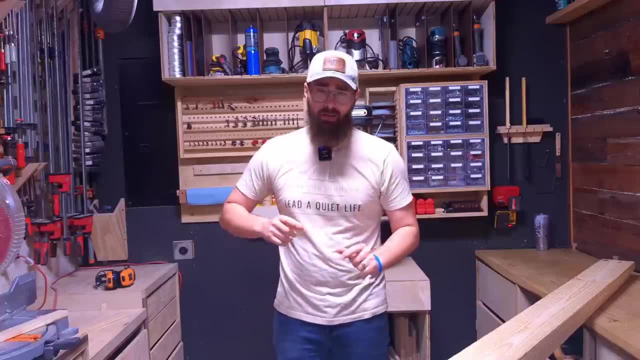 providing as much value as I possibly can. The plans will be made available for free on my new website here within the next couple days. Like I said, I will make a post with an update. So when I make that post you should subscribe so that you're. 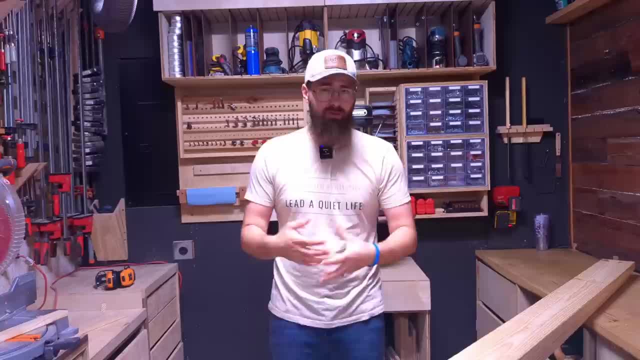 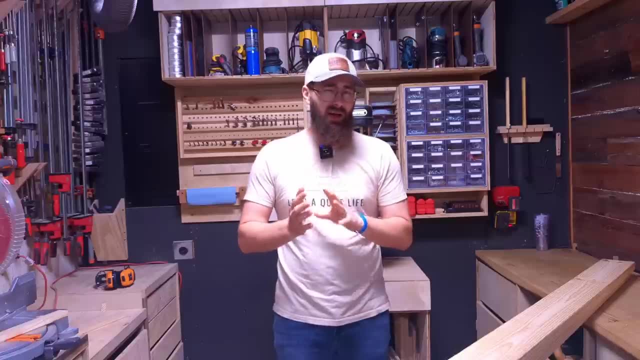 notified and you can immediately hop onto my website, get the plans for free and get started. There will also be an option to subscribe to a newsletter. I will be doing a newsletter kind of bi-weekly One. it'll sit out as soon as I post plans on my website. you will automatically. 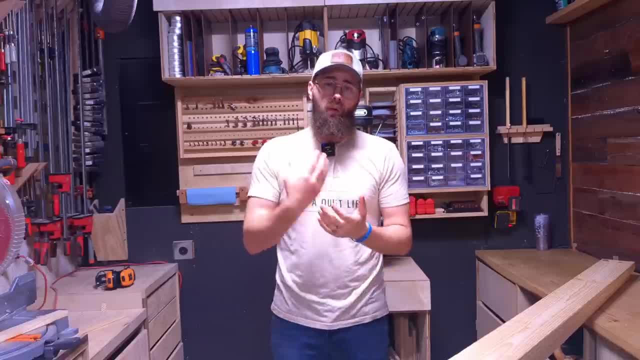 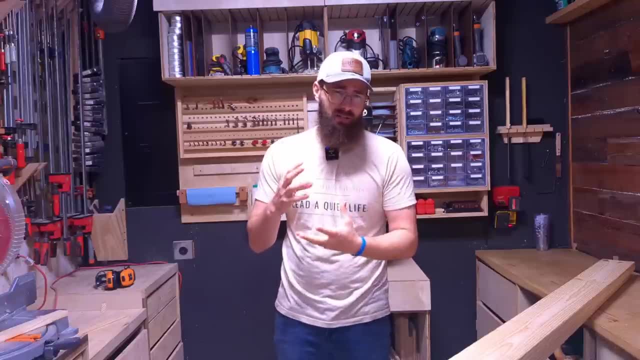 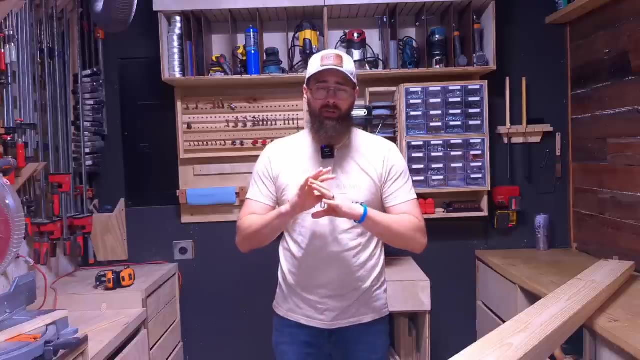 get a copy of the plans. There will also be some educational type articles that I'll be sending out. I have a lot of research I've been doing lately and I'm looking to make that into an easy to digest article format. I'm going to be sending those in an email, kind of a bi-weekly for now type thing. It's completely free. 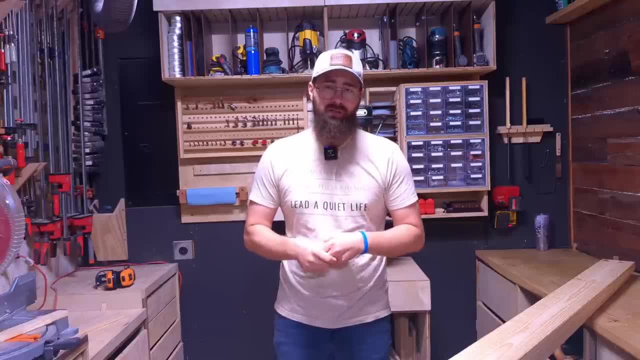 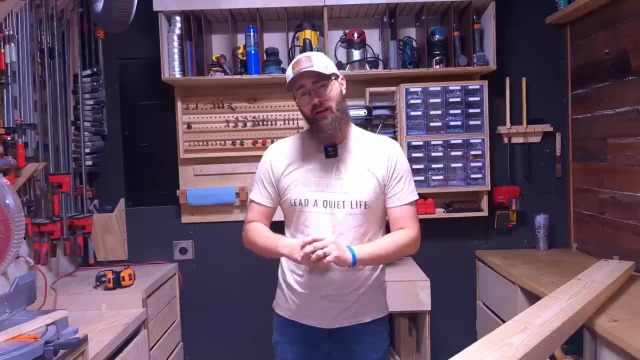 There's no cost. I don't get any of your information except your email address. Like I said, you'll get the plan sent to your email. You'll get the article sent to your email. It won't be spam at all. I can't. 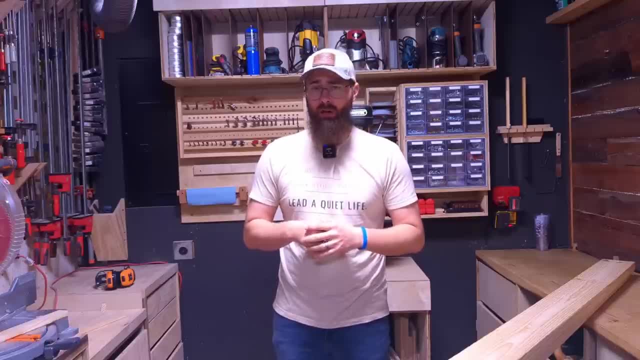 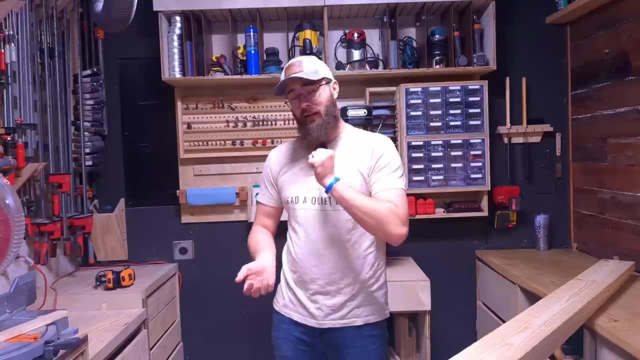 stand spam. I'm not going to spam you. I'm only going to send you stuff that I think is valuable, and I'm going to send it to you for free, That being said, like subscribe. Thank you so much again for the support. I am looking forward to. 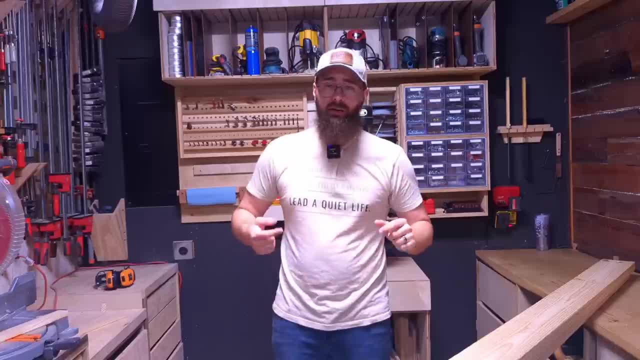 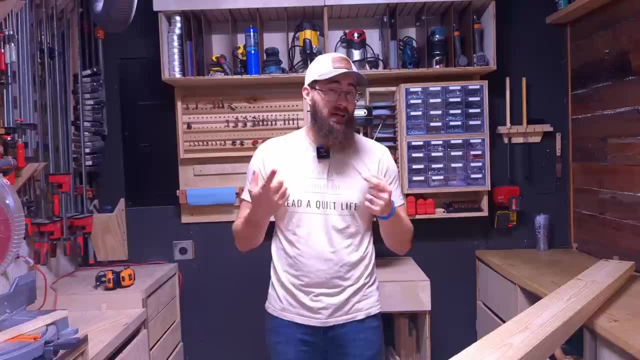 seeing what this channel does. Leave a comment. Let me know what you think. I am working on the plans for the next video as well, and I'm excited about that because I'm making a project actually for myself in the next one. So before we go, one thing, one last thing. 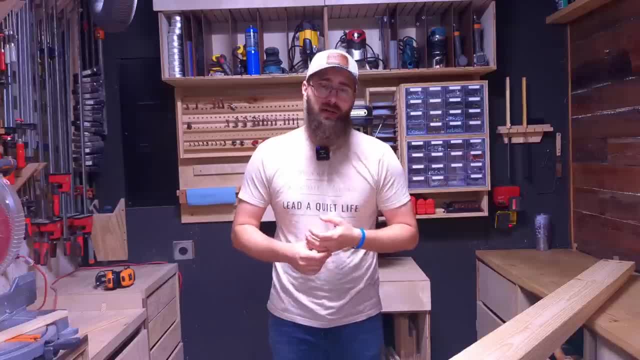 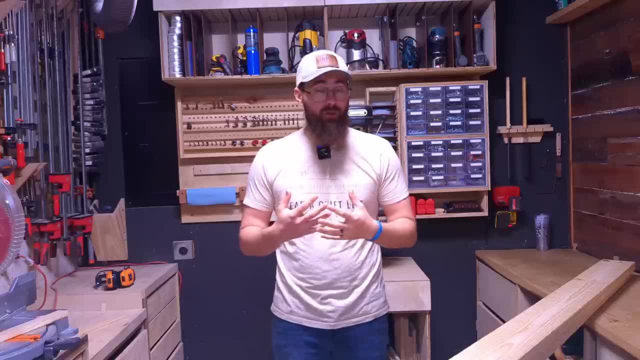 I want to point out I made quite a few mistakes on this build. The beautiful part about this build, the beautiful thing about beginner woodworking type projects or any woodworking project: it's okay to make mistakes. Don't be too hard on yourself. if you mess it up, Just make sure that you fix it You.